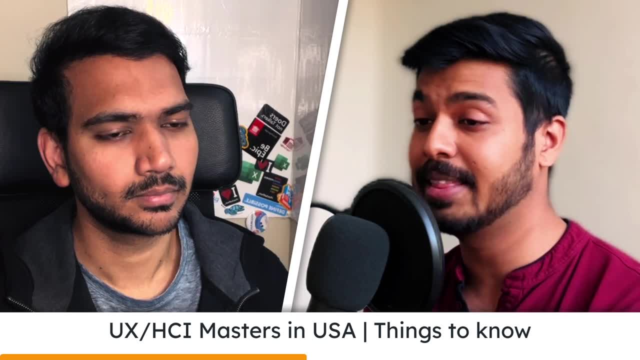 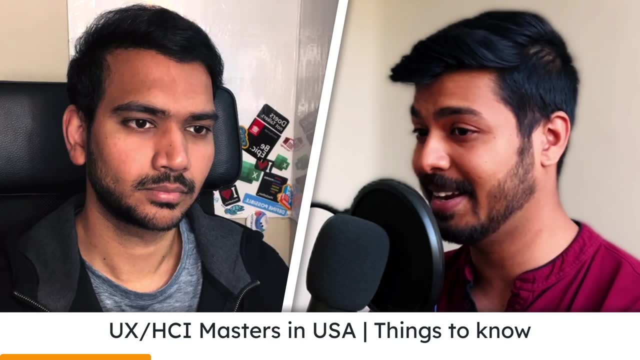 sharing his journey of getting into Masters and HCI in the US and then getting a job at Microsoft as a product designer, And also adding to it, Abhinav is my school friend and we have been to the same school back in India, and then we had to part ways for our different careers, but we have 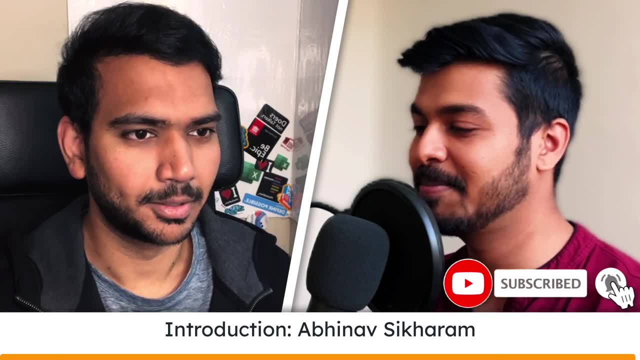 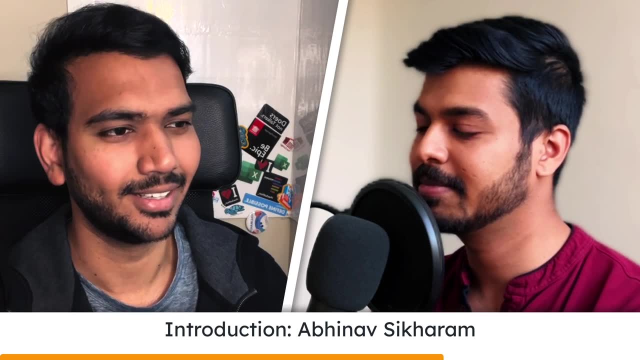 been in touch. So, that being said, I'll let Abhinav introduce himself. Yeah, thanks, Jofan. It's great connecting you to you back and we are kind of on the same field, like UX. It's really great to see a very close friend of mine, like being on the same journey with me. Yes, that being, 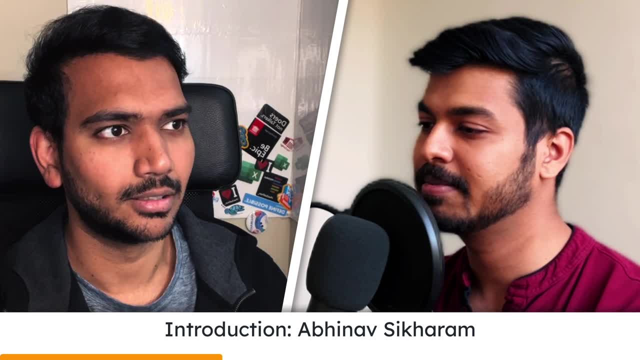 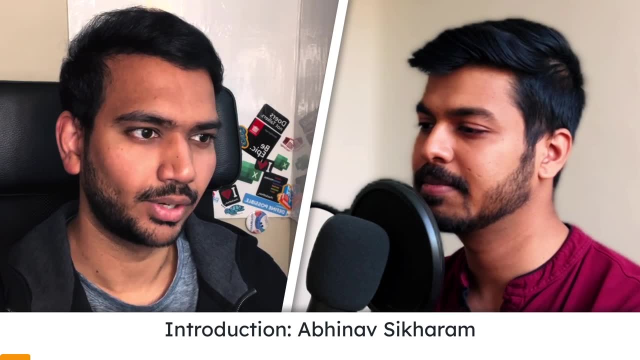 said: hi everyone. like I'm Abhinav Sikaram, I have been with Microsoft since last one year after finishing my Masters program in the US, So I'm currently a product designer too, at Microsoft in Office Apps. I'll move on to the next question. So, having a background in engineering, 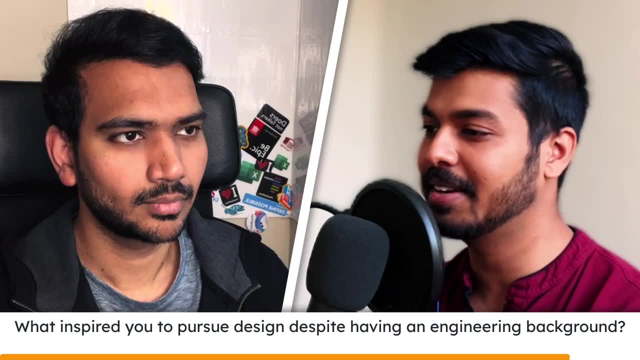 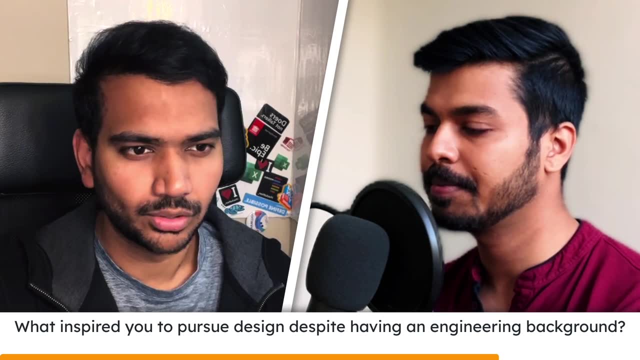 like, what actually motivated you or inspired you to get into design Back in 2013 is where, like, I had to give a class presentation on a new kind of technology. So that is where, like, I was doing some course out of internet research and ultimately, I landed up on a TED talk which was given by 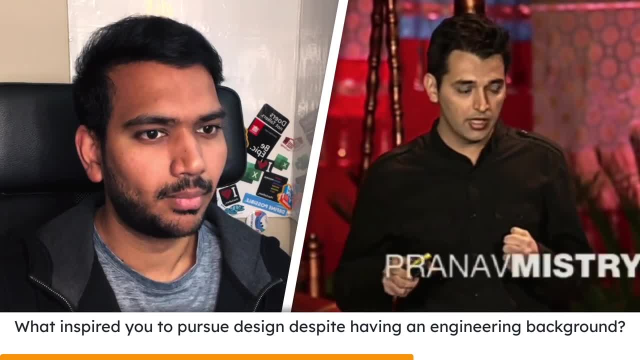 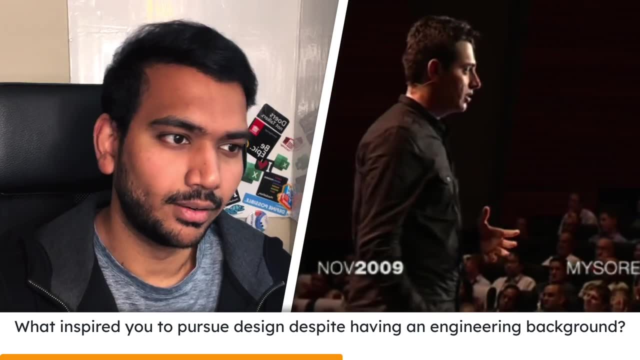 Mr B on a sixth sense technology. So, getting inspired by that video, I was trying to understand of what is his background and how did he reach that MIT BDL app, which was quite interesting, Like you know, the birthplace of bringing out the new technologies that we use today. 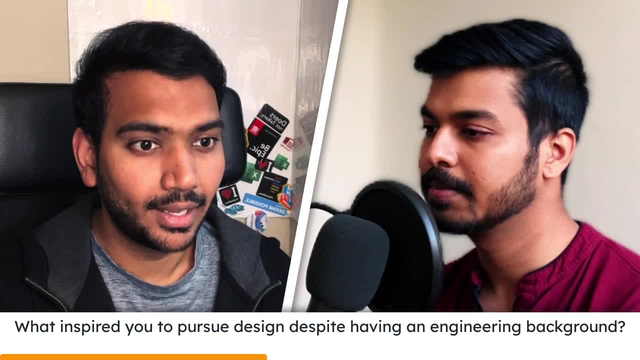 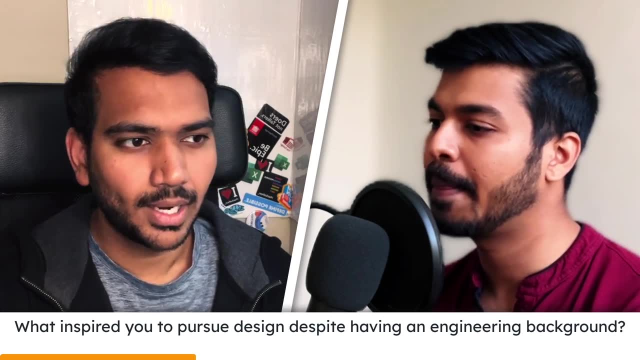 So, looking at his profile, and I did understand that there are design programs in India So that were offered by IDC, Bombay IITs and like there are a few IITs as well. Coming from that engineering background, this is something that I've explored all by myself at that time And the exposure towards 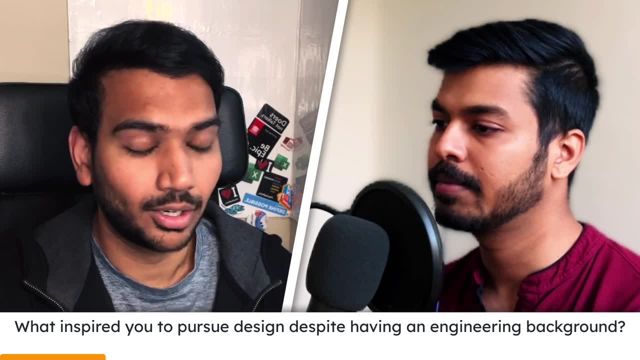 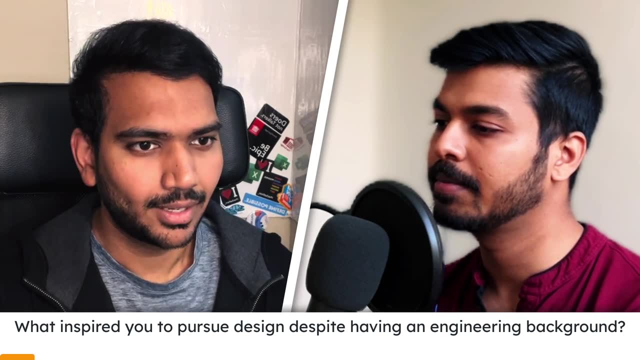 the design wasn't that great in 2023, or 2013,, but now it's kind of evolved. That's what I can understand. So that's how, like, I kind of explored the field of HCI. That's where the journey actually 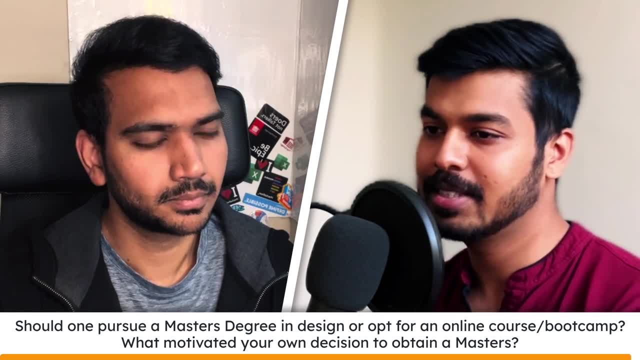 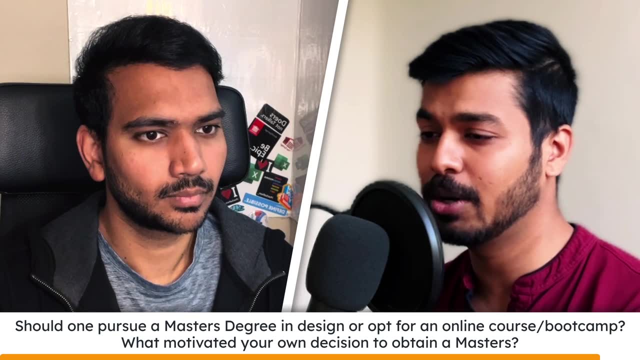 got started. So, moving on to the third question, this is a very common question that I've been receiving from people, whether they should get into a master's design degree or they should just do some online course or a boot camp. what would you suggest them, And what was your rationale behind your? 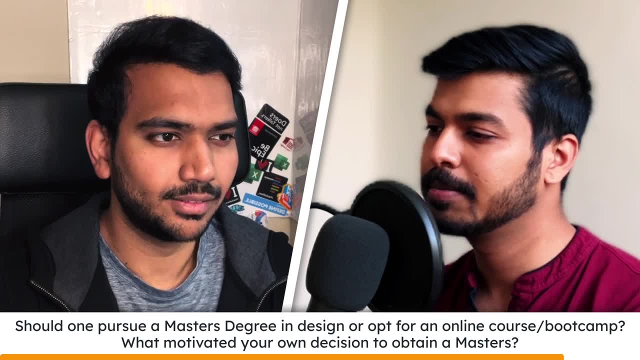 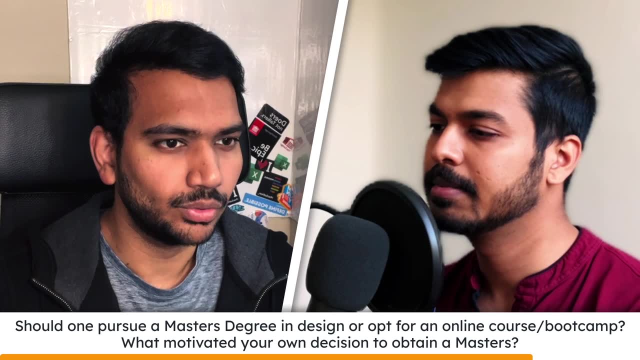 decision of getting a master's. As I've just mentioned about the seat examination, I didn't give my seat examination and NID exam as well For some reasons, like I couldn't make it to the schools directly because, like I did, stood at. 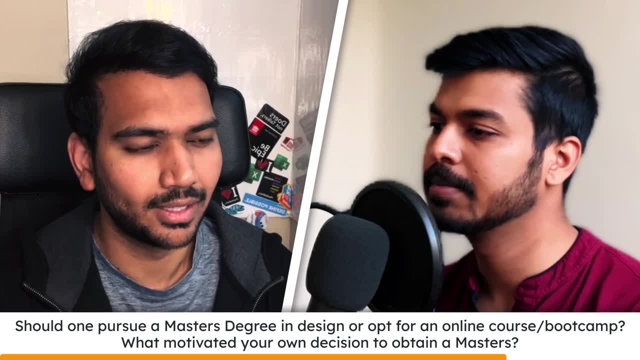 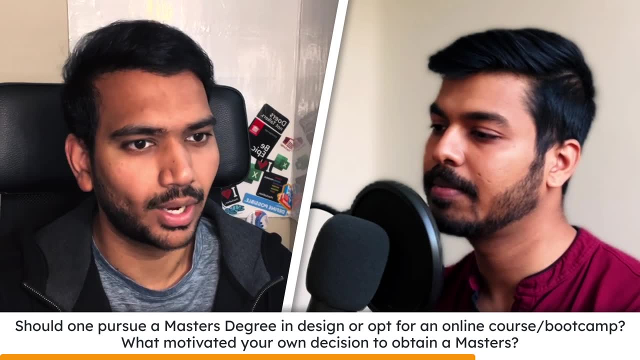 15th position, where there were only 12 seats and 90 seats. That really kept me motivated to say that, okay, I really want to have a formal design education before I actually can like shift my entire knowledge base from engineering to design, Because engineering is. 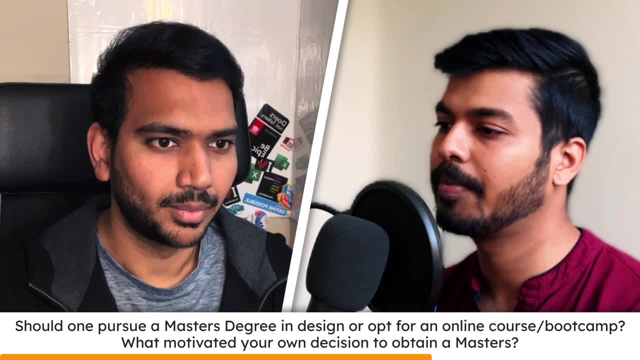 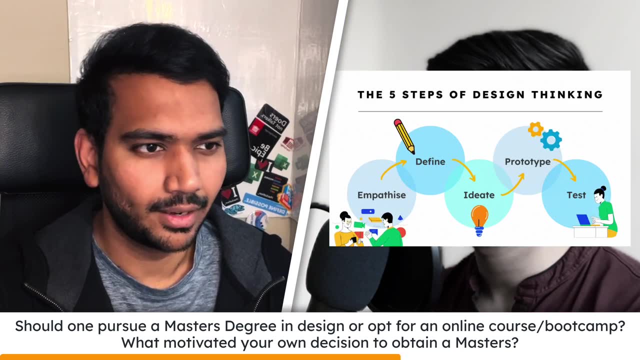 kind of different that we actually get out of that school. So it's something that is coding and something that can be manufactured or made out of it. But the process of design, the whole iteration like ideation, designing iterations and everything, and this is something that doesn't. 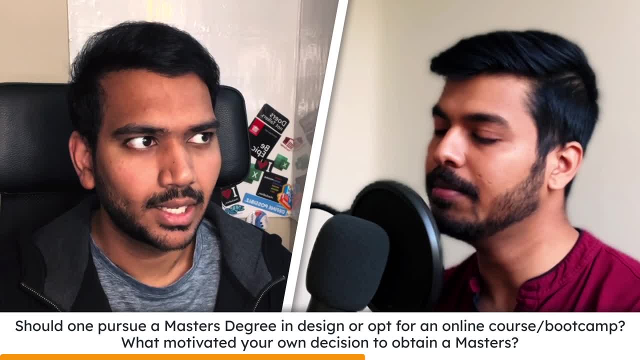 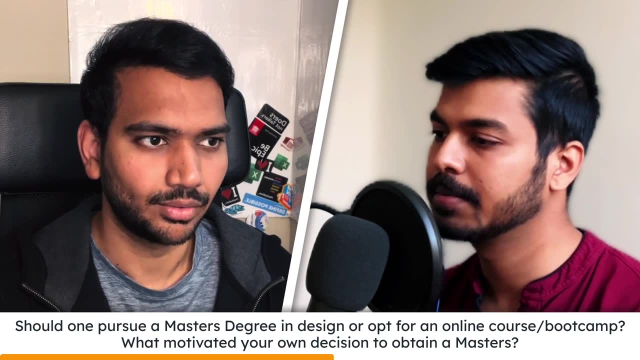 like really explored in engineering. So for that I kept thinking that I might need a proper design degree or at least a master's program to get into that area itself. So again, when I was trying to understand this whole area in 2015,, 2016,, there were 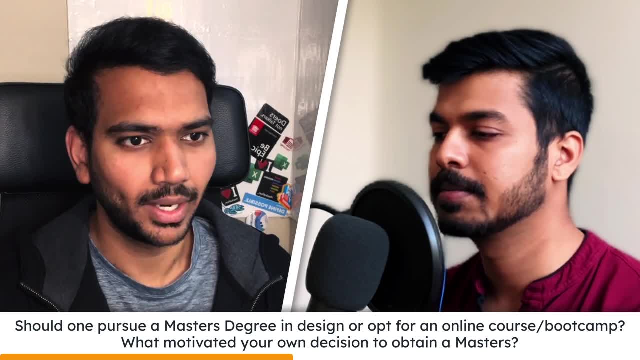 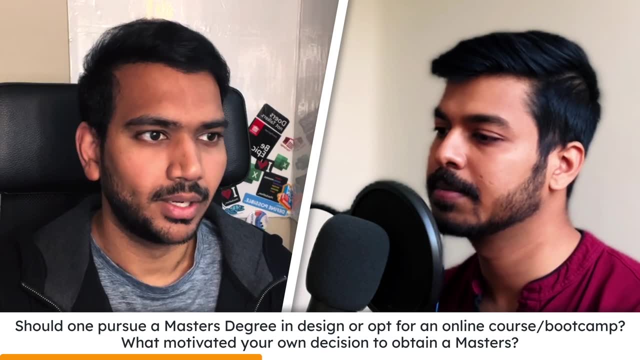 much of these boot camp programs, especially in the field of UX, The only entry point that I could find out is mostly through NID and seat examination within India. But yes, as I couldn't make it to those schools, that is where I kind of also found. 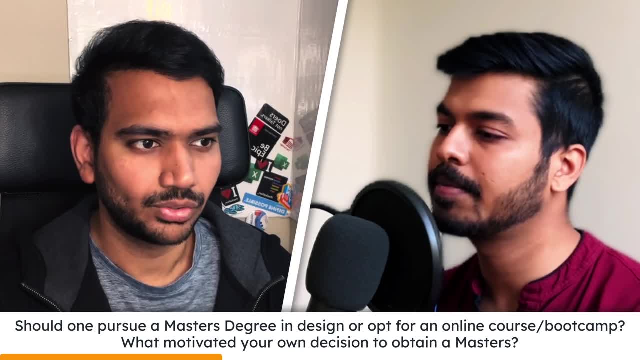 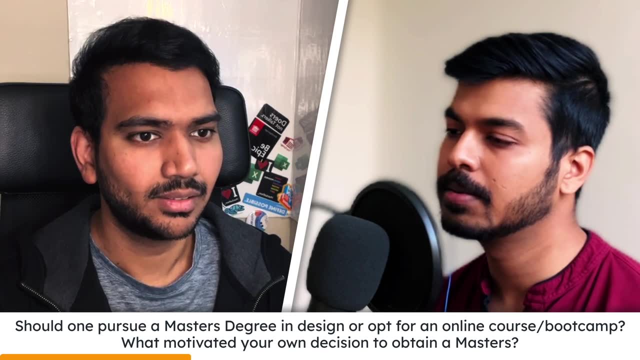 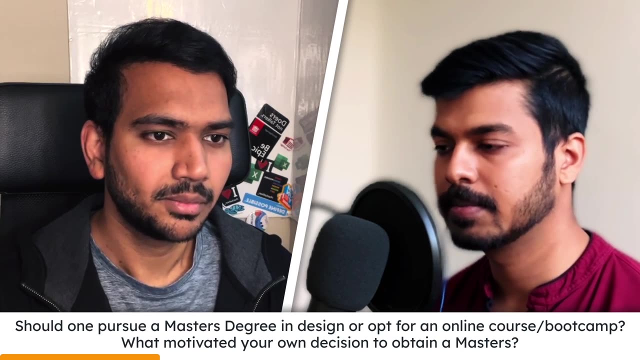 this massive open online courses like from the edX or course setup are kind of offering these kind of UX programs and the product design programs. So I did try to understand of see if this is the right thing for me to do- And that is where I started- to a product design course from that university based in Netherlands. 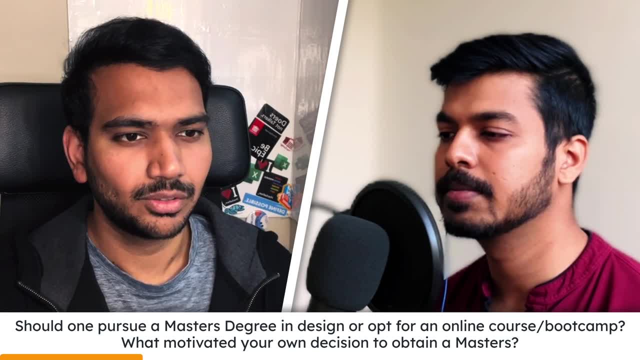 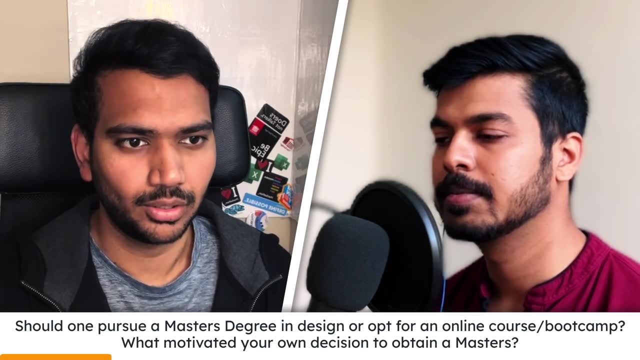 through these edX platform. So that kept me interesting. So it was a six month, six month program. So I did finish that course And I didn't really feel that okay, I have learned the basics. I've understood the what is what in the 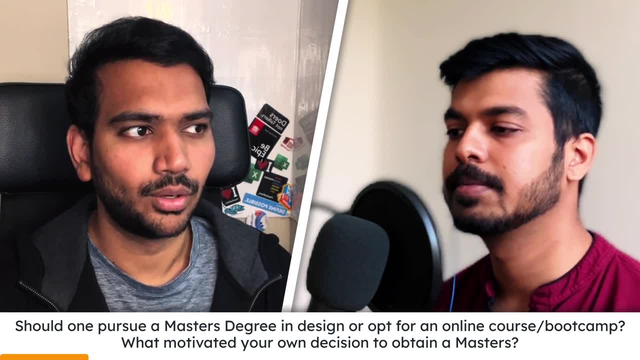 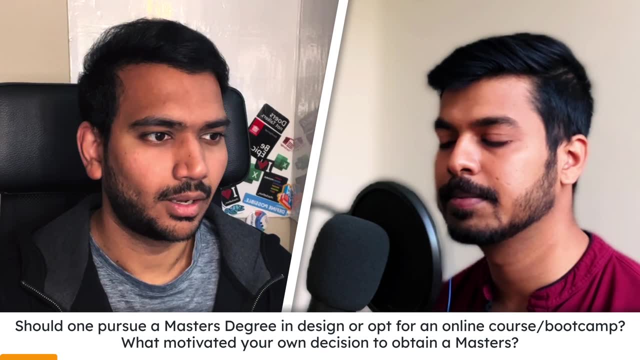 field of design. but still, I didn't get that confidence in myself saying that, okay, I'm really capable of giving an interview and aiming for a UX, a professional UX job itself. For those reasons, yes, and I was working in back in. 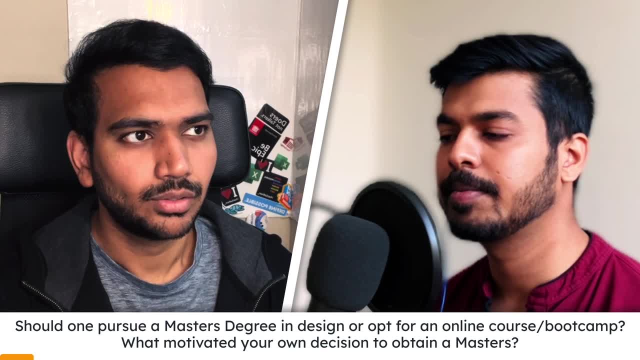 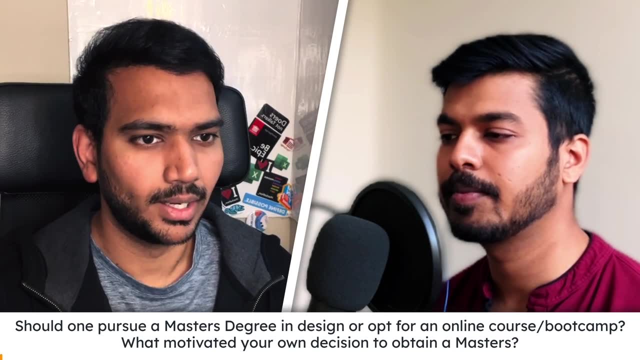 Cognizant for three and a half years like a programmer analyst. So that is where I kind of understood that, okay, I need to understand design a little bit more from end to end. For that reasons I need a formal degree. 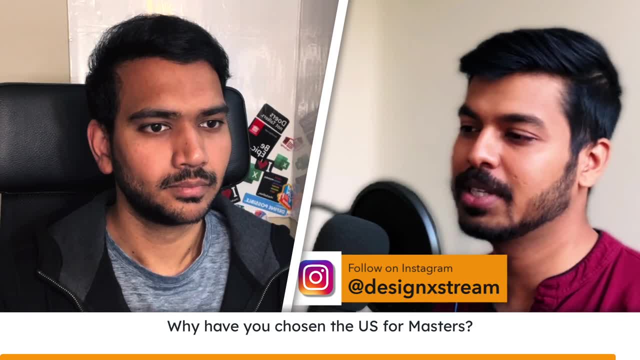 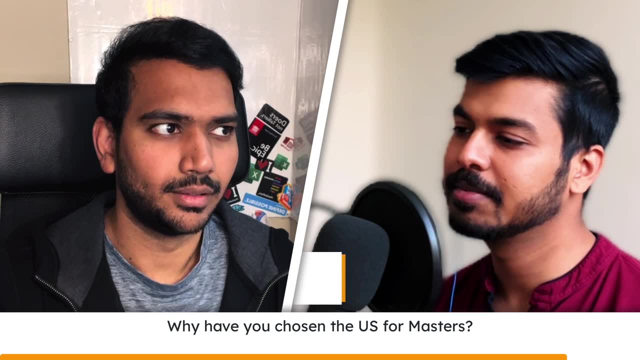 Moving on to the next one, like: why did you specifically choose us? Why didn't you choose Europe or Australia in the other country? But yeah, it's kind of a thing that we, at least in India and India has this. you know, US is a go to thing, But yes, I did. 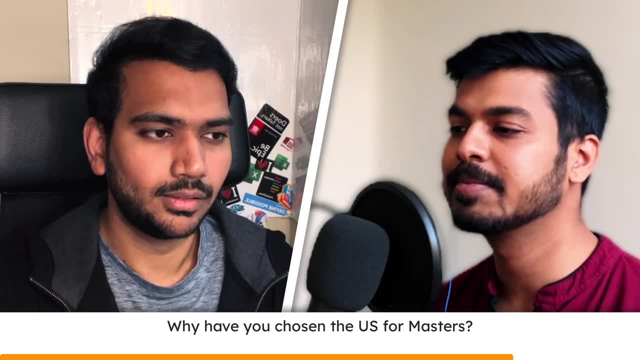 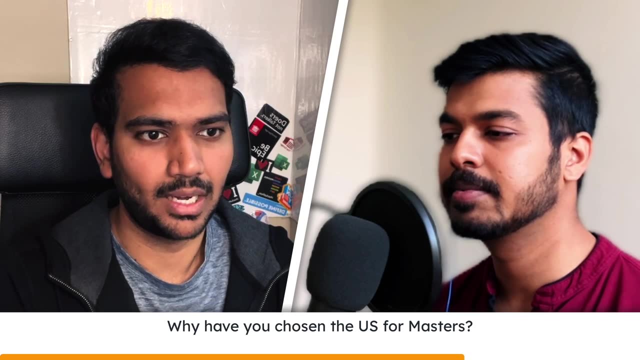 consider some of the others just in Canada. And I did consider the University of Delhi because, after taking that edX program- like you know course, why don't I choose Delhi to Netherlands? because that is kind of the program that I really. 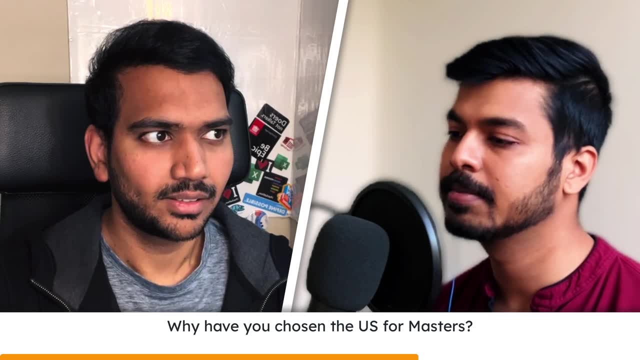 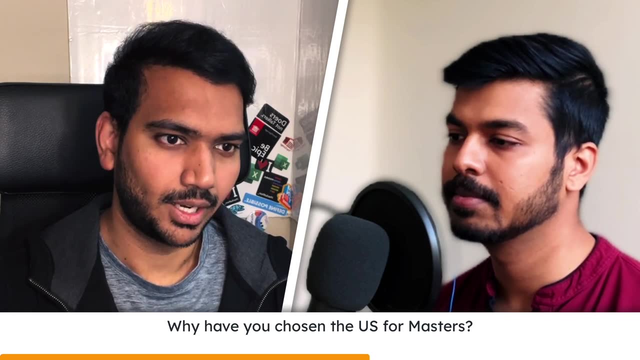 wanted. It's kind of a personal choice that I could say on one side. it's kind of the first place, as I've mentioned, like MIT Media Lab was the first school that I've explored in that very first TED talk. So starting from there, like I was trying to understand of what are the 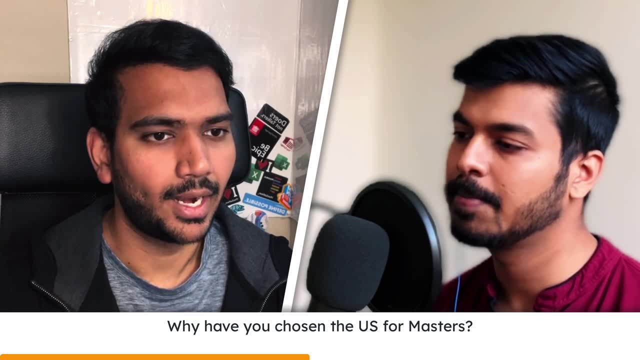 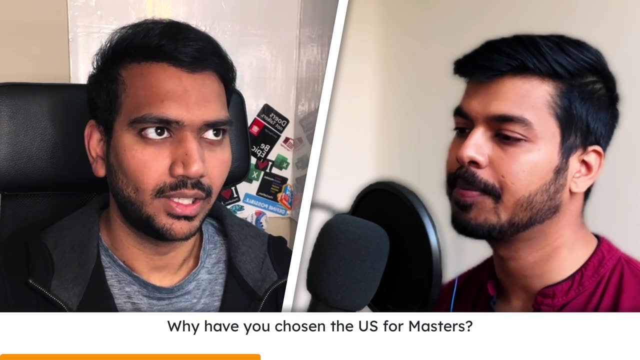 different universities that are offering these six year programs and how long they were into this. you know research and design side of it, So that is what I could see. that, okay, US is a place where I could professionally explore a much bigger. 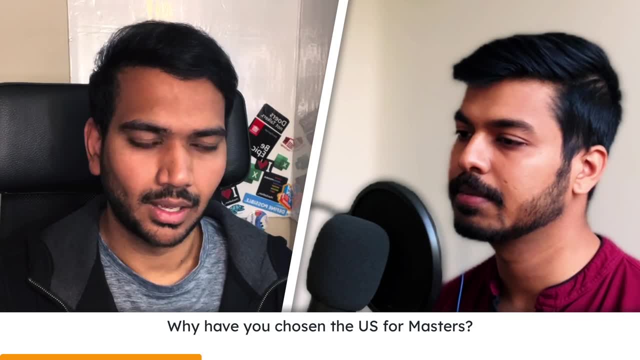 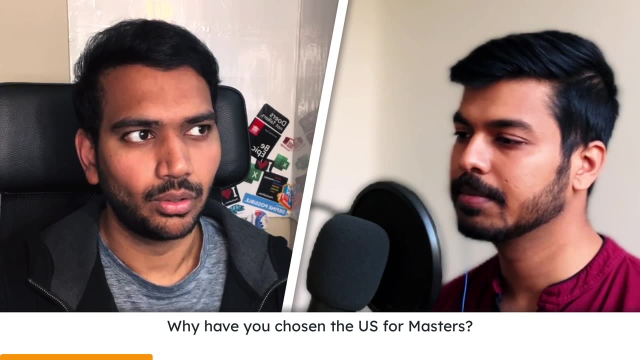 head's yet, because that's where the whole new things are kind of popping up, And so that's the reason like I have opted these for the US, But again I do suggest people to look at for Canada as well, because Canada is also having the start universities that offer the 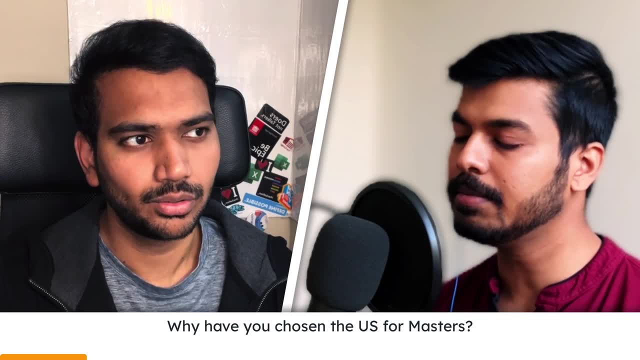 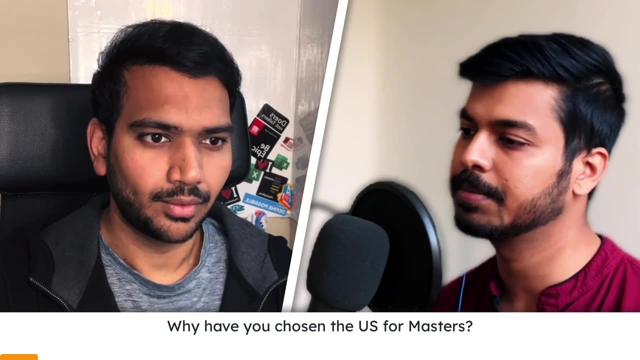 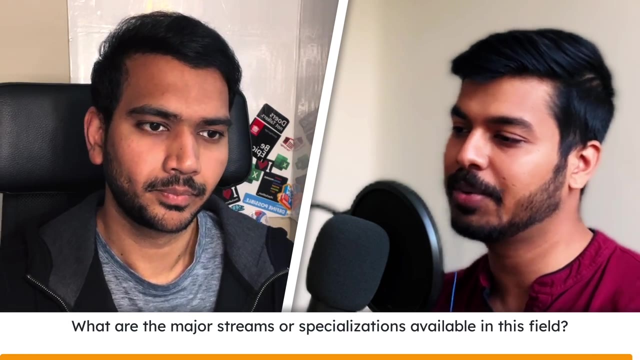 strong head CI kind of men. when I say strong head CI courses they are into PhD kind of 11 courses because they are into complete research And I do have few connections where they are into the complete head CI research based on. for a person who's not aware, like let's. 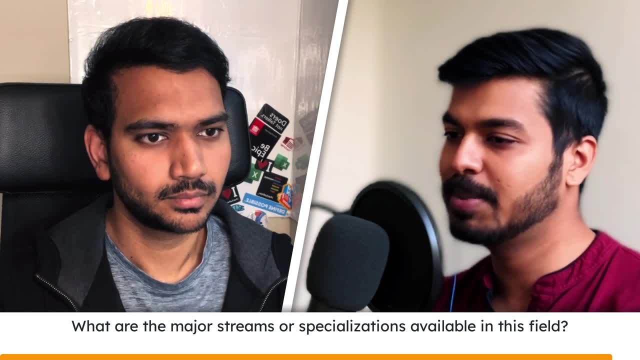 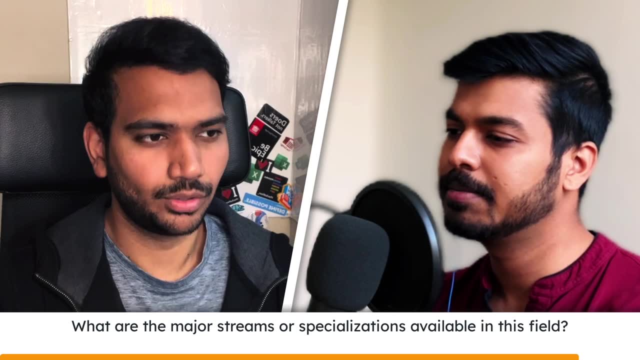 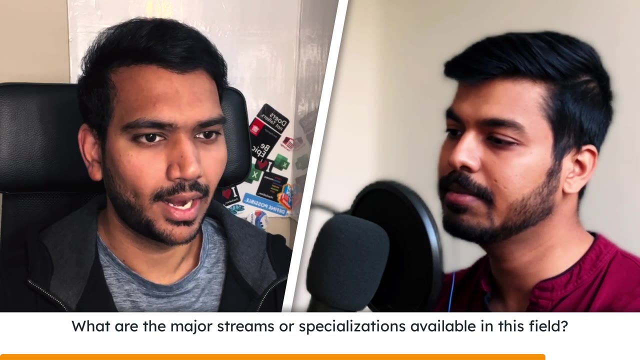 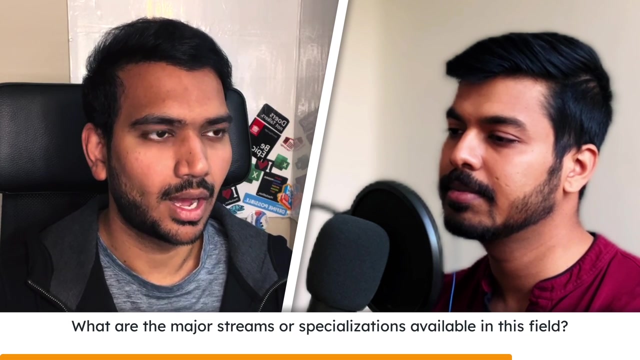 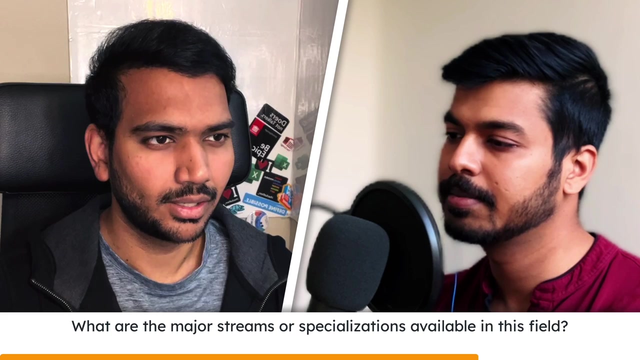 say they are in their engineering or doing some other degree. What are the specializations or you know degrees that they can look into to get into UI UX? So yes, when we talk about user experience UX altogether, it's kind of a very broad area. So when I say very broad area, it's something that your passion and your career options, where you want to actually set it out or think of it like again within UX, we call our designers at self like a simple designer for interaction designer or a product designer or industrial industry design is kind of a completely different thing. 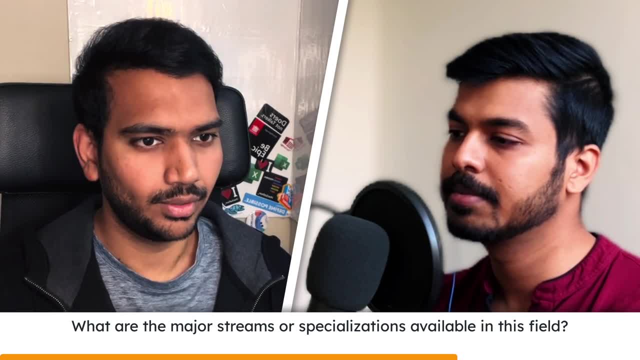 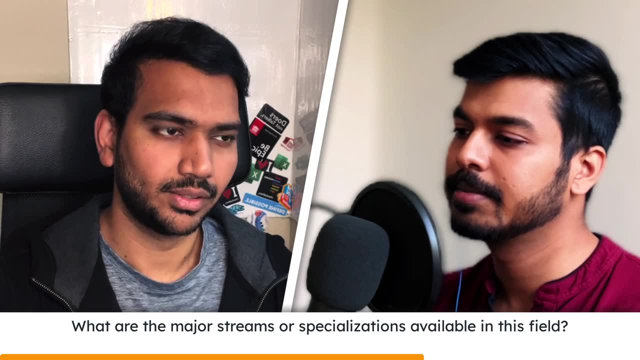 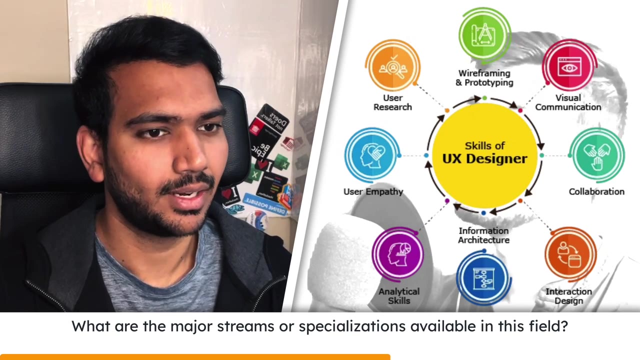 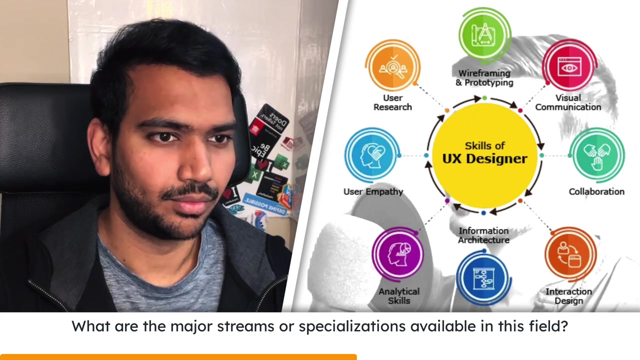 But, yes, industrial designers aren't called product designers And we ourselves also calling ourselves as, like, a, product designers, like we do on the software side of it, but they do on the hardware side of it. Okay, so you have different streams itself, like even Accessibility is one of the designers, like even there are Accessibility designers who are specifically like or specialized into those designs, and you have audio designers and you have video design and so on. you have illustration designs and you have, like visual designing. 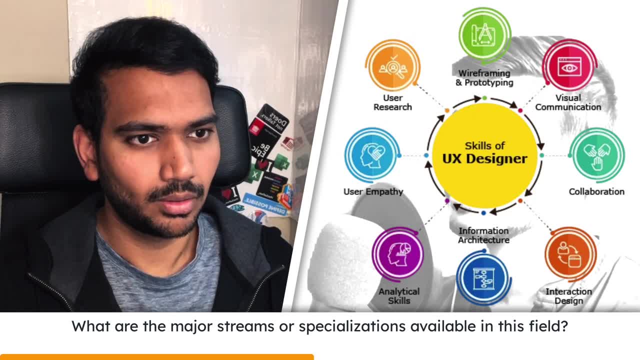 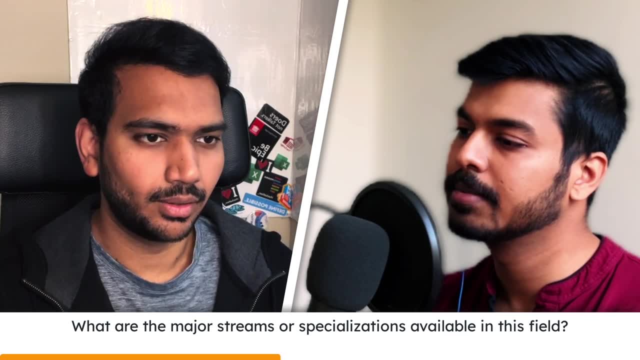 Yes, there are different. like LV was called a designer. on the end of the day, like visually I'm kind of a little weak, while I can like strategically add, like when implementing from an end to end flow, like I can work on those core concepts, like kind of the engineering stuff. 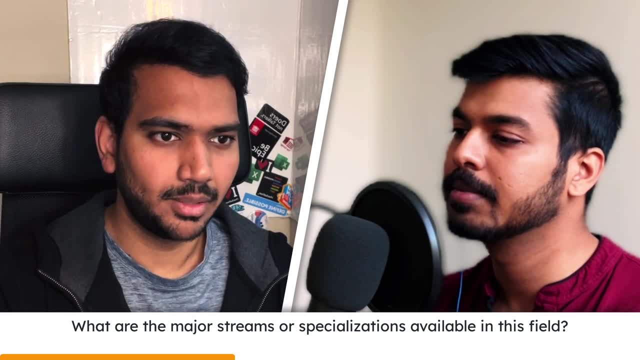 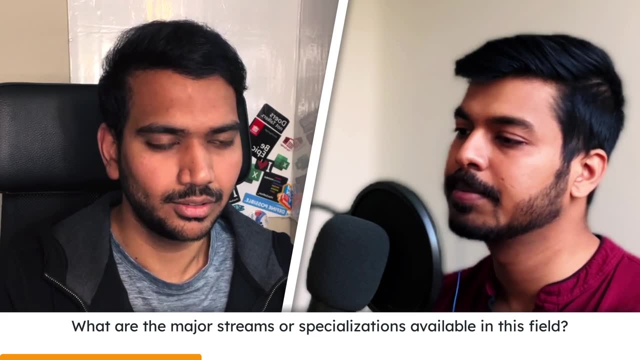 But from the other side, another person can actually could actually be very good at like visually. you know they can be representing their art like art form on the kind of create the illustrations, but they are kind of strong on the visual side of it. 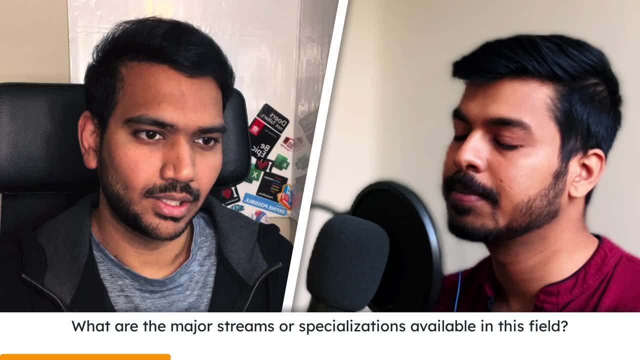 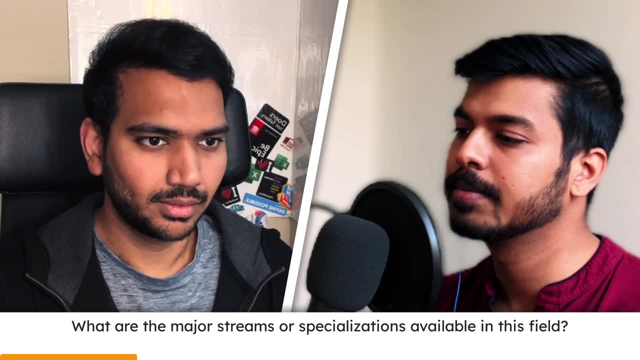 And they might actually need to like come up with these strategy tool learnings of how to create those interactions. So it's like we need to put ourselves into different spaces within the UX, learn everything from end to end and see and explore all these areas. 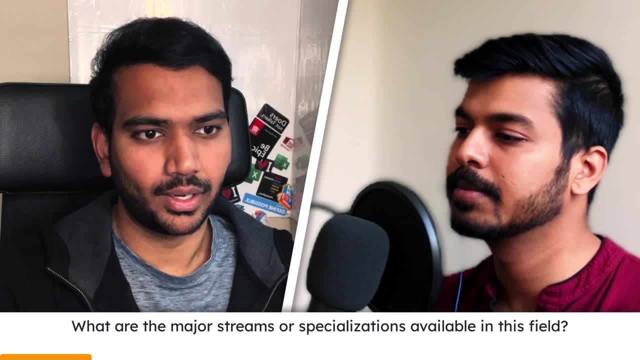 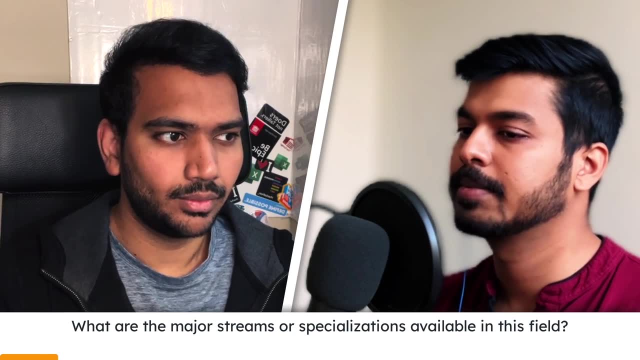 And then ultimately settle down at one area where they would really want to work and, you know, become more kind of unicorn within that particularly So it's like when you're in the early stages, it's better We hustle around these kinds of things. So it's like when you're in the early stages, it's better, We hustle around these kinds of things. So it's like when you're in the early stages, it's better, We hustle around these kinds of things. We hustle around these kinds of things. 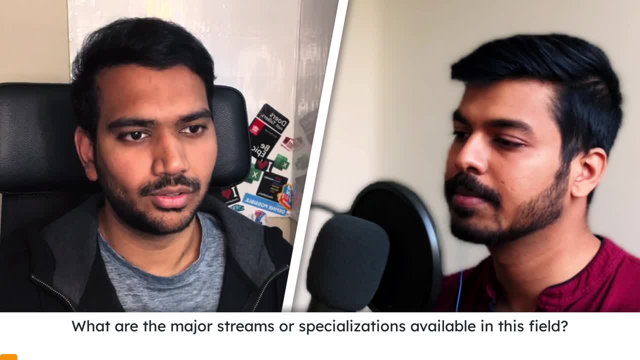 And then eventually we can figure it out and we can understand, like what are the strong areas above the areas that we need to improved and perk? And then eventually, we can figure it out and we can understand, like what are the strong areas above the areas that we need to improved and perk? 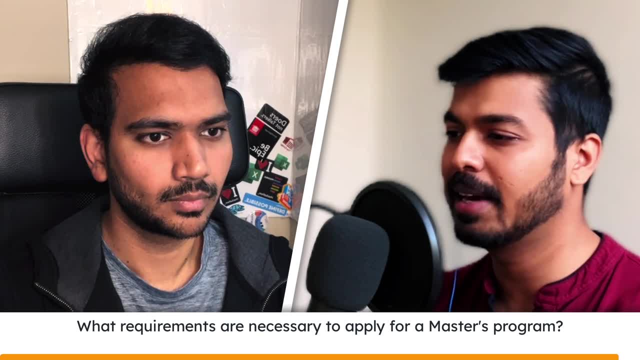 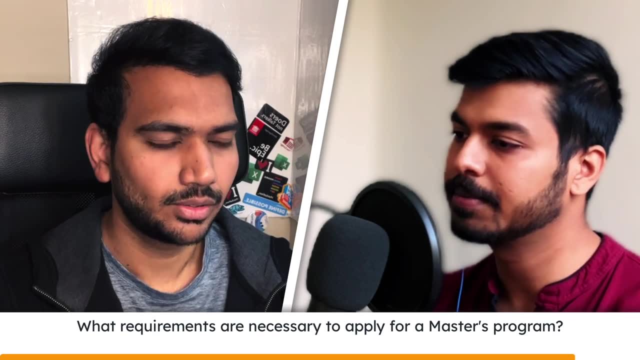 What are all that are needed to apply for a master's program. let it be like the eligibility or the portfolio, like what exactly is needed. It's almost the same in India and in the US. we just need to clear the basic exam, entrance examination spells. okay. 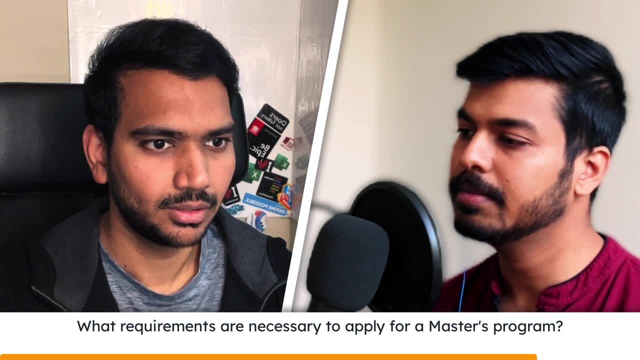 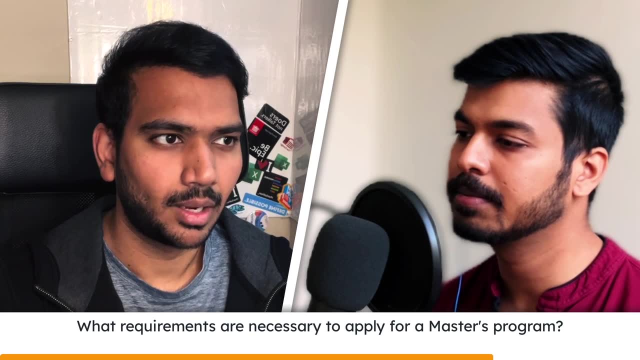 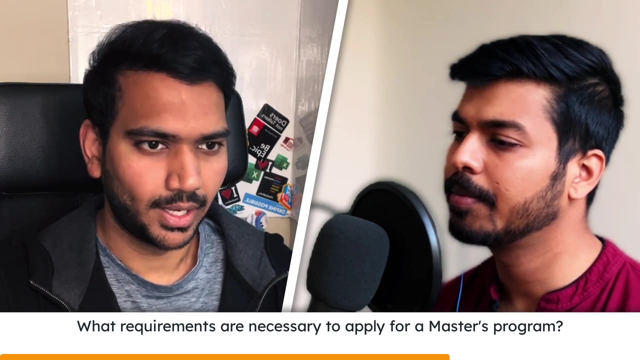 In India. it's just like SEAD or NIE examination and once you clear that examinationyou will be given a call to all get into the interview. so you'll be having- i mean, different schools- interview you in a different base. so, yes, you need the seed exam, national identity exam, and you need to give that internal 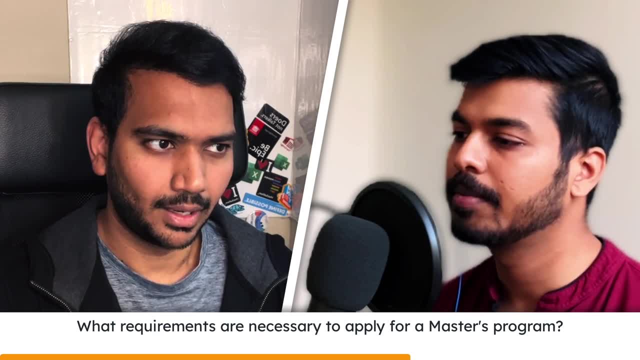 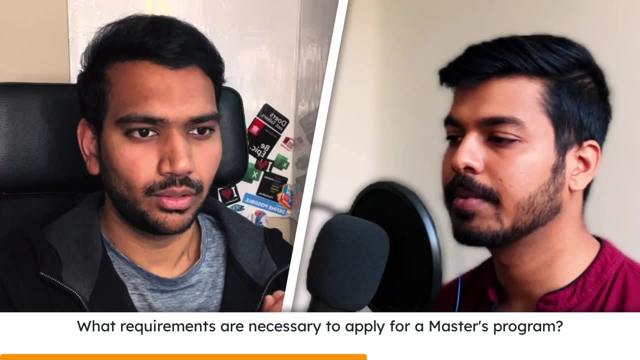 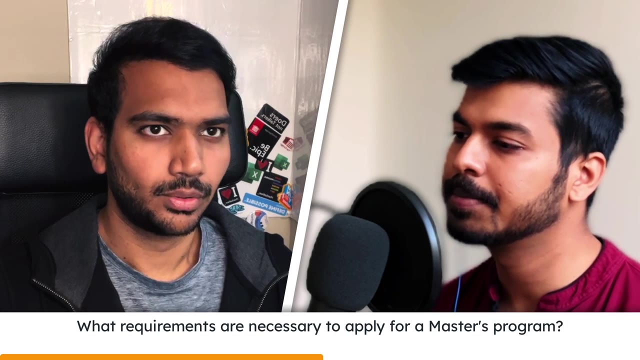 exam where you go on site and you give that attempt correctly and at the same time you'll do well in the interview. so all of these schools accumulate together to give into your final score and getting into a seat, and so that is the process in india to get into a master's program. 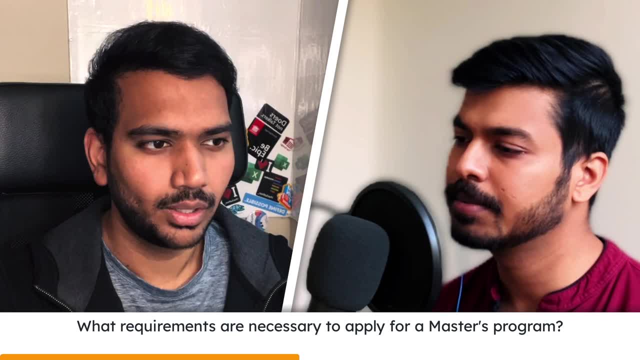 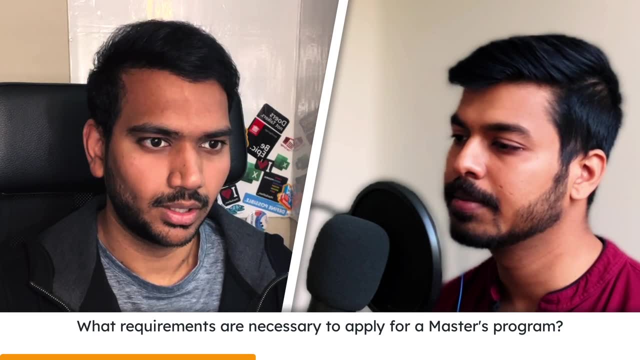 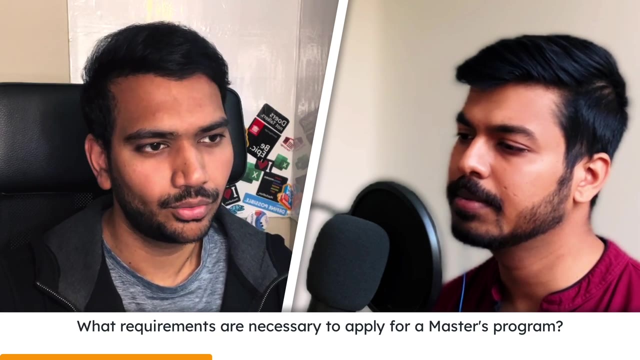 uh, when coming to the us it's it's only a straightforward process of everyone does that. uh, you need a gre score and you need a TOEFL or IELTS, but english fluency kind of thing, and the next thing would be a portfolio. i mean, most of the schools would ask you a portfolio. 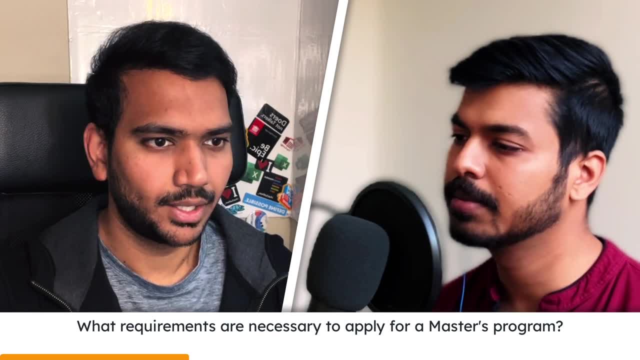 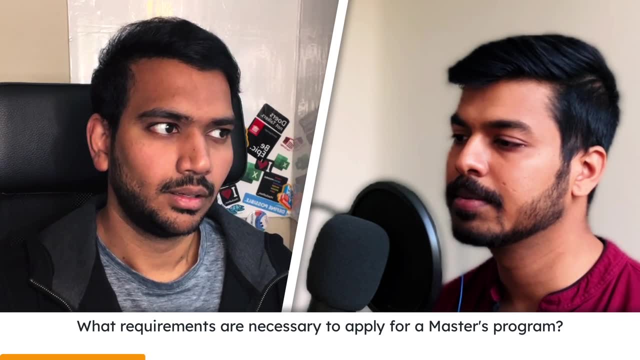 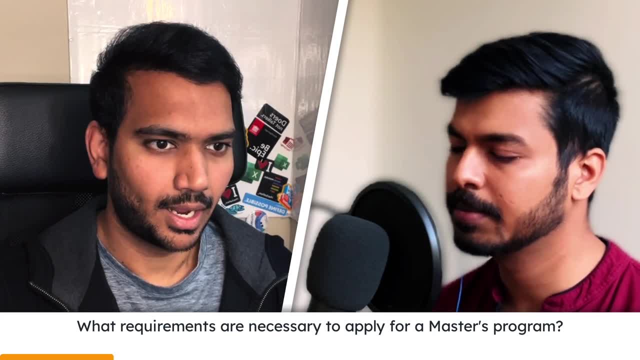 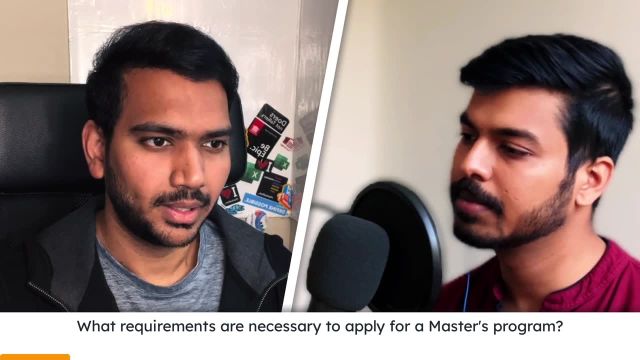 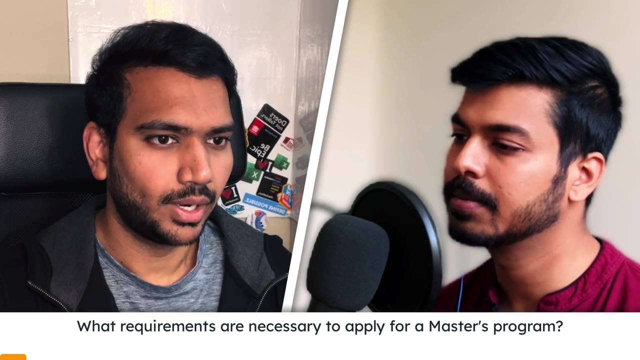 in 2019. i just had a pdf portfolio that i had and just uploaded it. so, being having a strong sop and having a resume that actually talks your interest with that portfolio, it could be a pdf portfolio as well, and a good jre score would end you up on the good universities in the us. 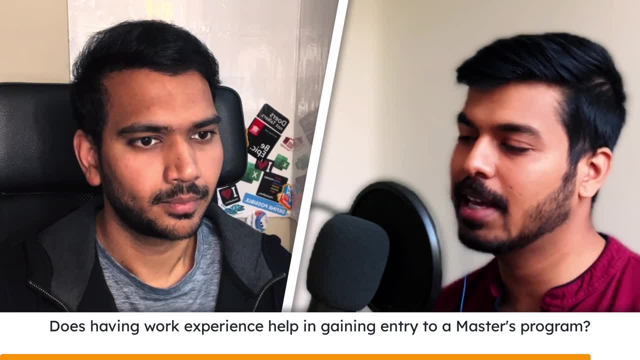 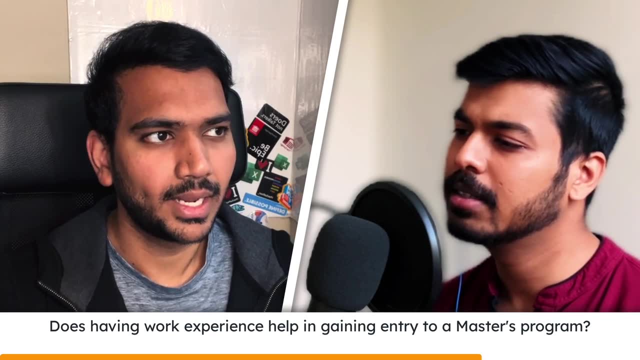 one more additional question to this: does actually having an experience help or a beginner, like after completing your engineering, people can jump. does that add as an extra point if you have experience? well, in my case it was like i worked for another company. again i'm back in india like for concept technology solutions for three and a. 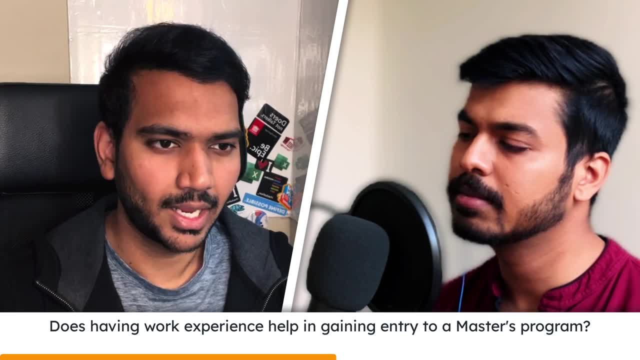 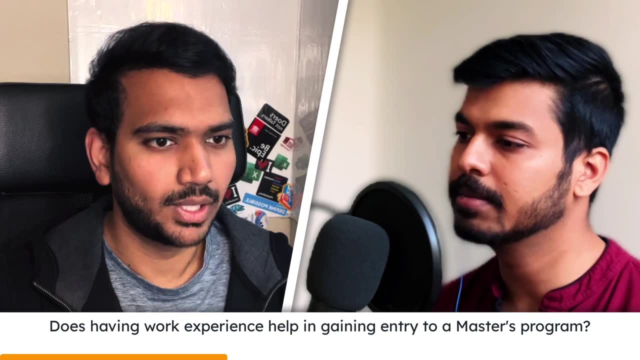 half years when i'd say yes and a no, because i have seen my peers who have just completed their bachelor's again and into bearing and not just required in design and most of them have ended up, you know, coming to the nci program straight away. so getting that in the 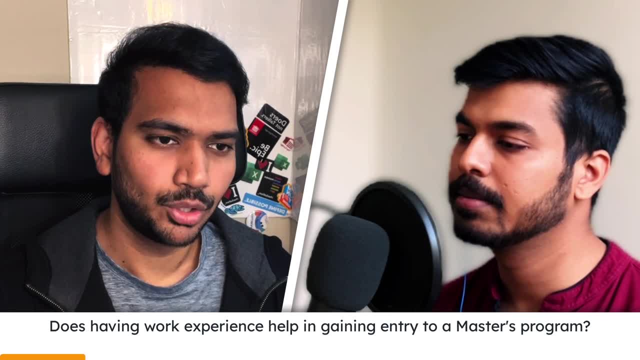 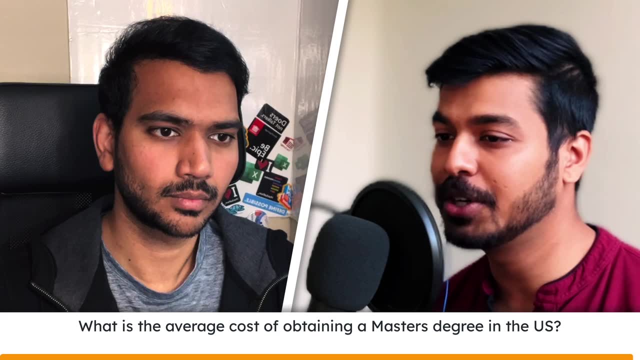 industry exposure is definitely going to help in getting into an internship quicker and better internships and as well as a better job. that i could say on average, how much would it cost to get a master's degree in the us? i mean, it would actually cost you a lot. that considered to be the 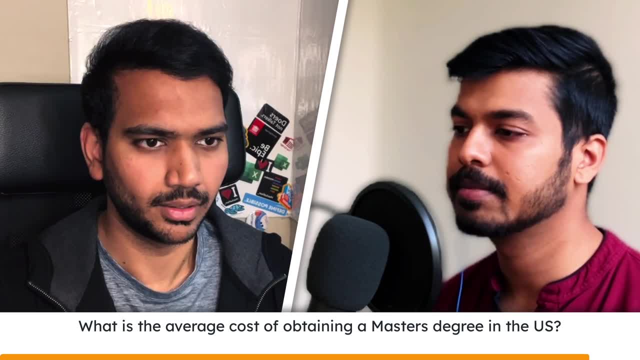 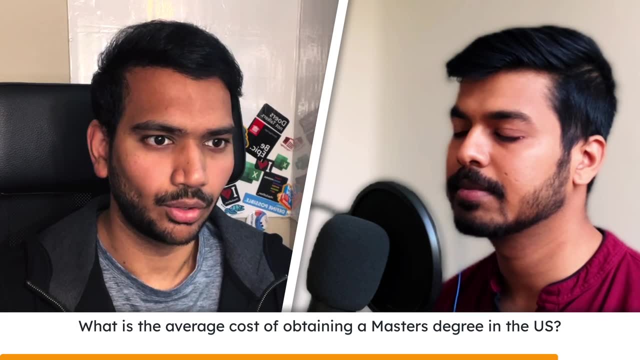 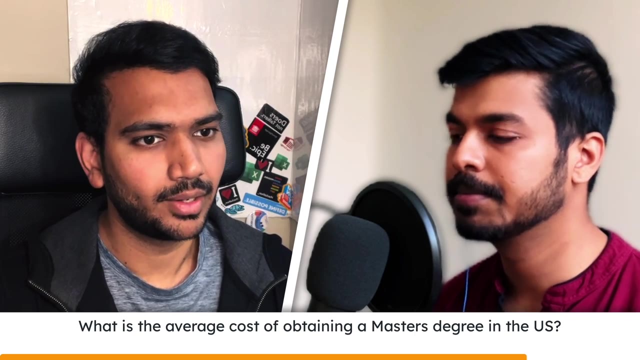 top tier itself, like even in the field of it's here for tellers. so getting into those schools need a good jrs course and good exposure on what we are going to do or make you know who you are going to work with in within that university. i can't give you an exact number on how i really 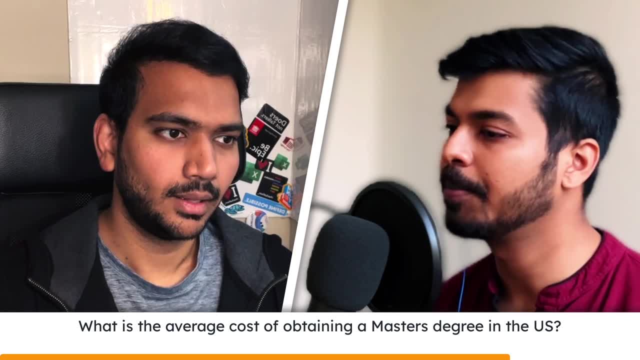 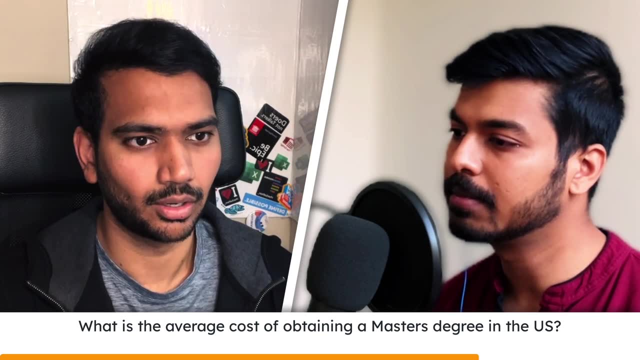 caused, but they are the costliest. it's in the us. then next comes the pilot universities. i can't apply to one of those universities and got an admit to it like it is a college student district of technology, rit and upstate new york and it was costing me around like 16k. 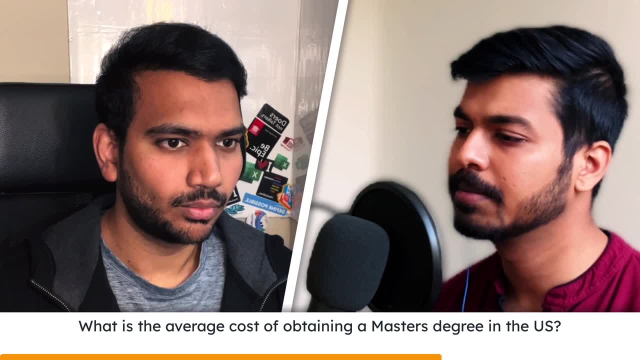 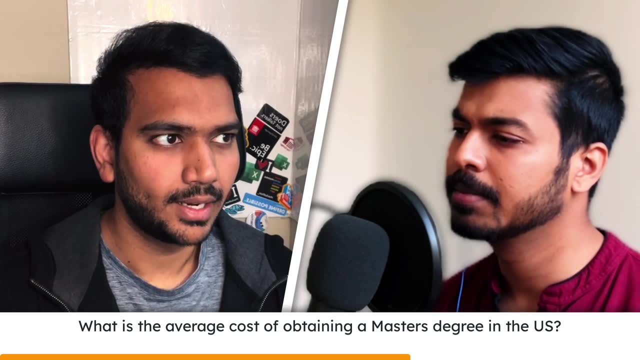 us dollars like for the two years program. it's considered to be one of the best programs within the university it started in the you know in the us of for its year. but i can't they've seen like i did apply for iupui like indiana university particular university in annapolis as well. 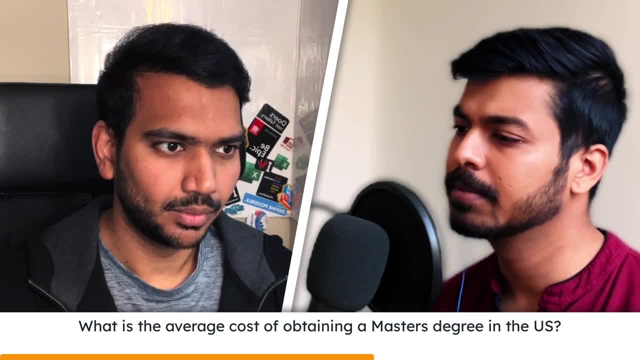 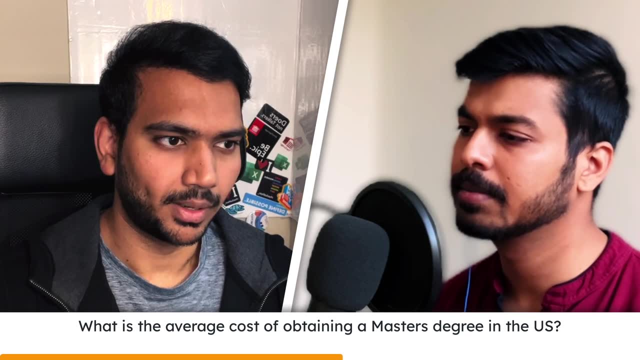 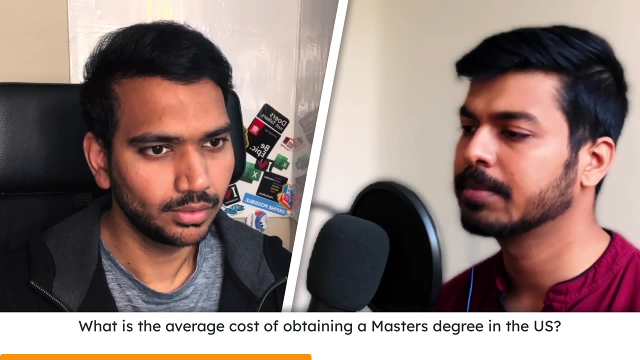 which is a public university and it is kind of a decent university, which gave me a scholarship and which gave me an- uh, you know, dr, our research assistants as well. so, and it did cost me around 30 to 35 k us dollars, but, yes, for the next two years, so by years. the reason that i opted for iubi is 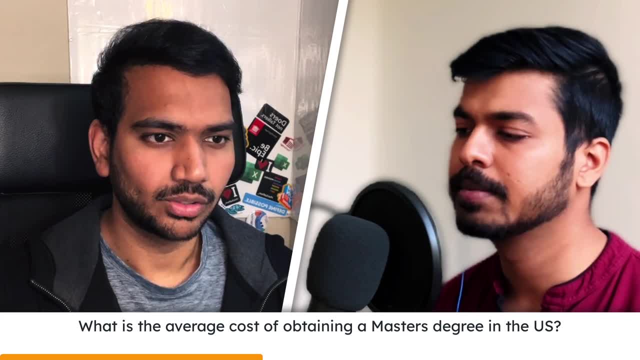 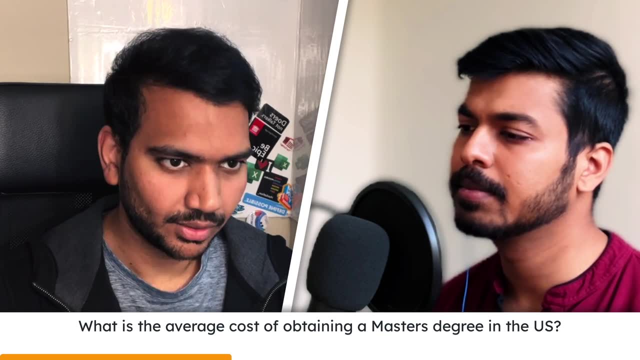 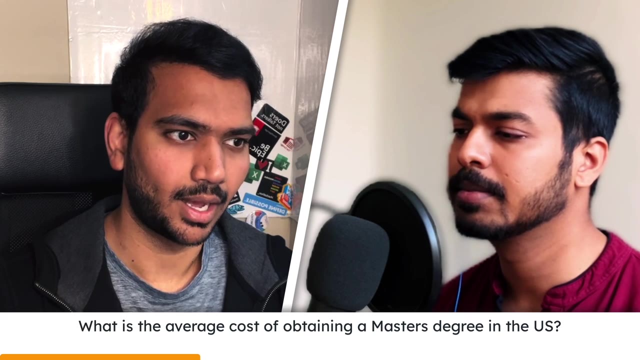 yes, one. it is being a decent university. it is not costing me a huge bucks. uh, you know, at the end of the day, i won't be on a huge deck. the second reason is i received a scholarship saying that, okay, this person can be given a scholarship for that, and i did receive a ta or a uh assistant. 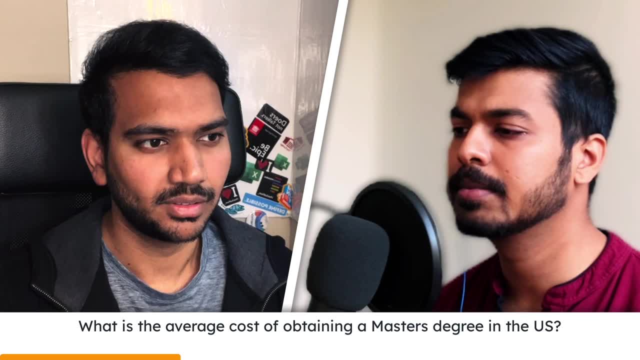 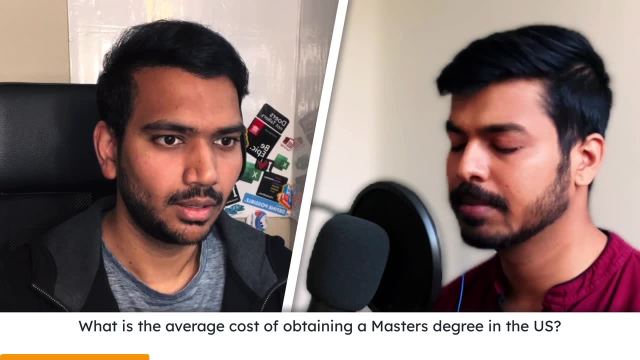 so teaching assistants are getting the teaching assistants or research assistants, is really important uh to not just getting the or, like you know, uh getting the money in it from it when it's that you get from the research and when you work with the professors itself. so, okay, do position. 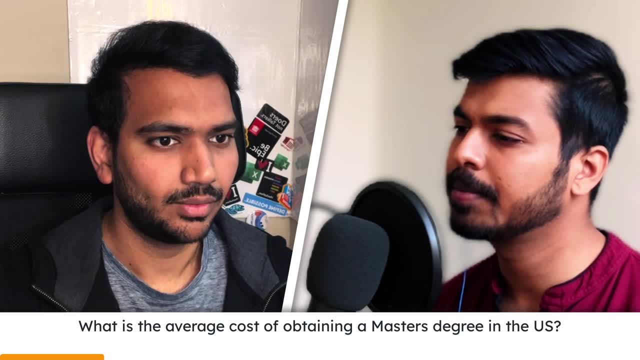 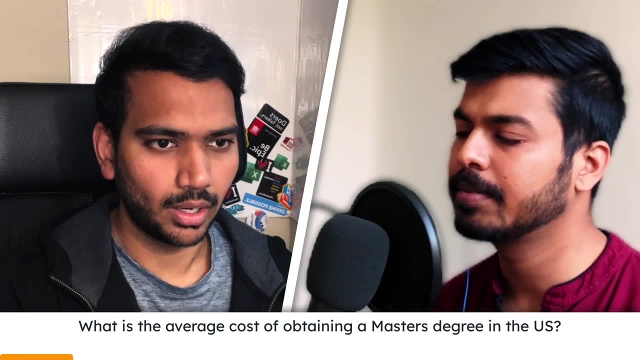 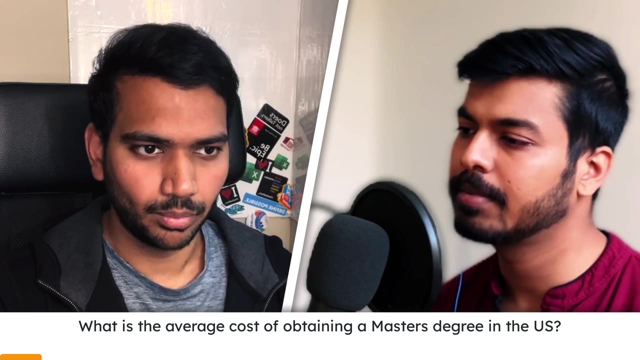 i mean, like i'd suggest, like anyone to position themselves and see, uh, if a normal university is kind of giving you all of these benefits and, ultimately, if you are aiming to reap the benefits from that particular university, and if you find out, uh, that they have good, good enough professors. 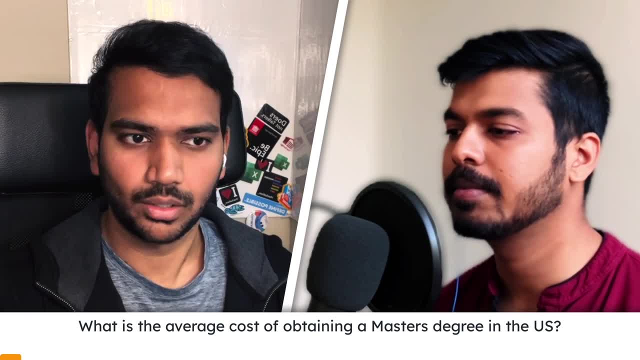 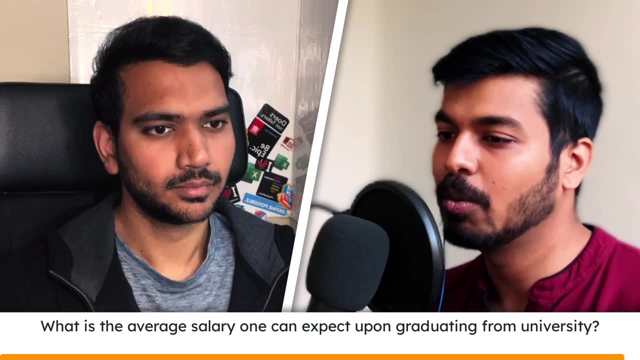 to back you up through learning side of it, i'd say to opt for a public university, because that's the safest fact that i could say of once you graduate out of university, like what is the average salary one could expect, and also as you keep climbing up the ladder, like how is the growth? 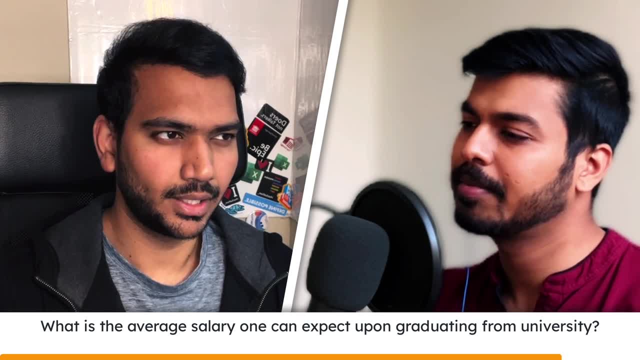 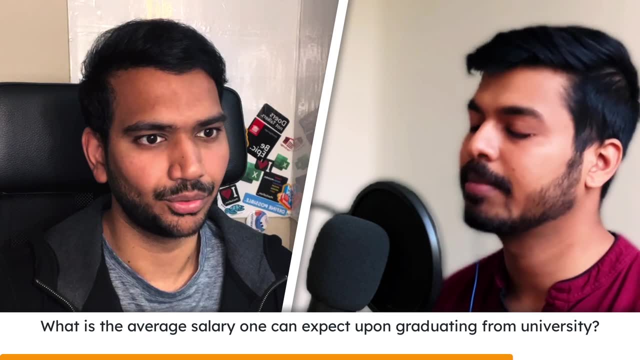 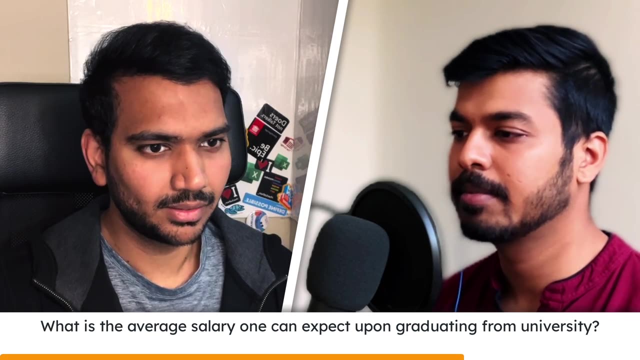 in the us. well, yes, i am kind of late early in the career, so behind in the us, right, so the us works in a different way. like the numbers are not straight away put out there. but yes, you can find the average ux based salary for that particular state. like it varies from state to state. like 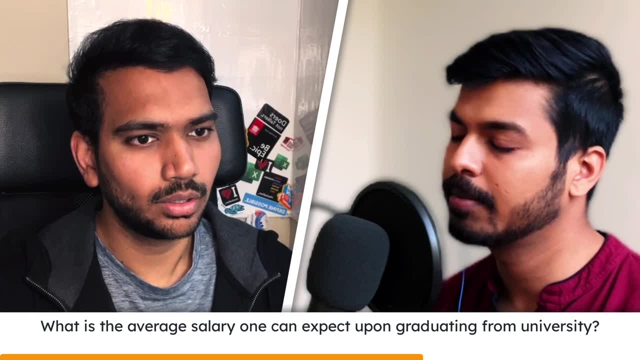 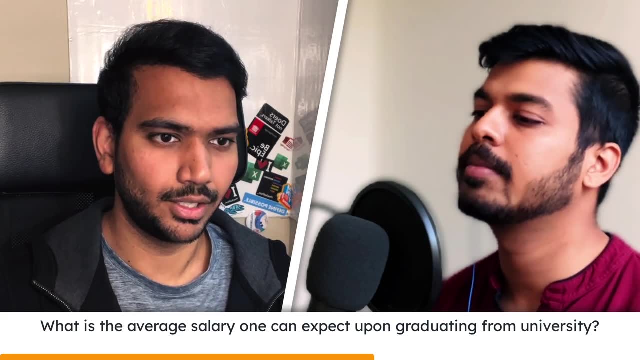 california is kind of repay kind of more, but compared to the state of georgia, like the way that i am right now, because it has different kinds of logic surrounded the living conditions or the living cost of living or whatever it is. so for those reasons, like if microsoft is, paying a same ux designer with an x amount of money in the seattle area, which is the headquartered area, i might not receive the same x amount, so it would vary within the company and within from the states to state to state within the us, so i can't give you the exact number on how it is. 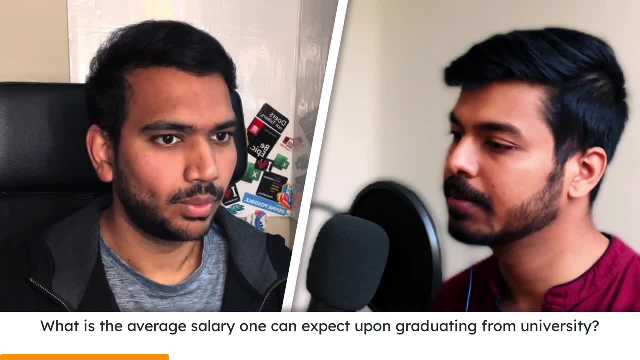 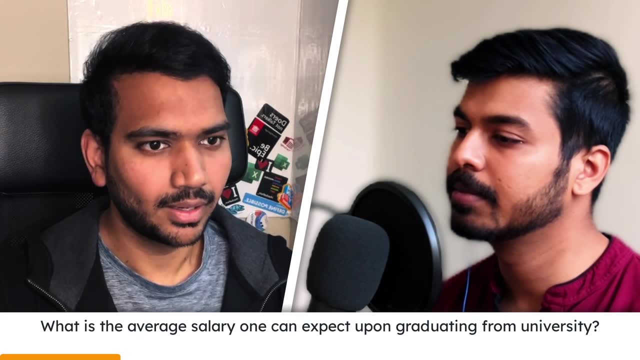 but what i could see from the trends recently is ux is a field that is going all together in all of these companies, just because everyone is trying to understand the importance and necessity of being the user advocate and user-centric and making user-centric products. so for that reasons, 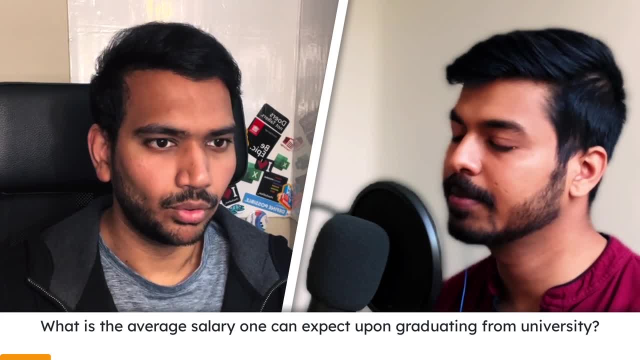 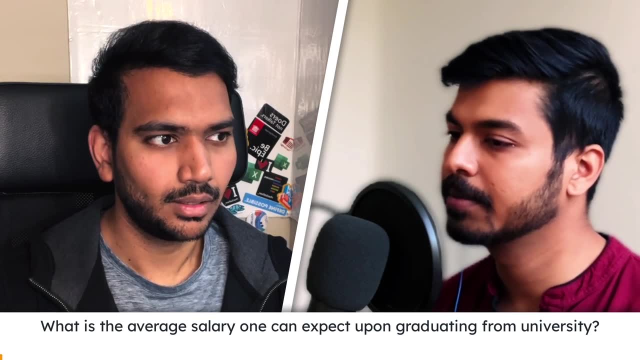 the trajectory of the growth curve is kind of improving altogether and you could see a real good growth in terms of salary and the packages that you receive over here. going on to the next question, i think this would be interesting, like how did you get into microsoft? and like how was 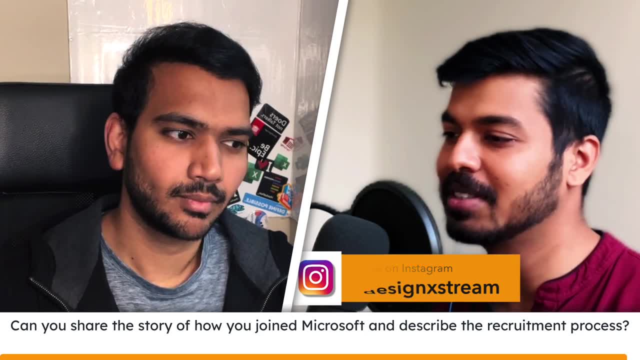 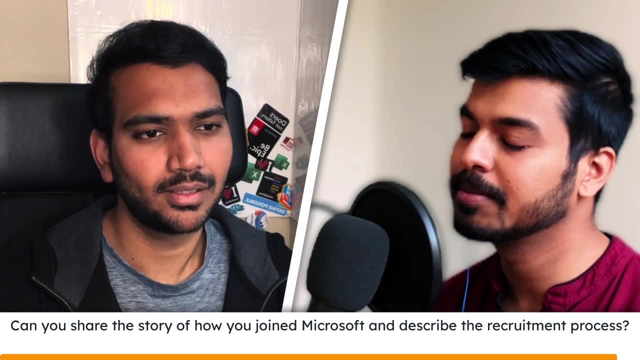 the recruitment process. like was it hard? yeah, like if you could give us a brief of it, it would be great. so microsoft is not like i. i never kind of aimed for to get into this fine companies as such, so it wasn't a thing for me. like, i need to get into the ux field. that is the whole. 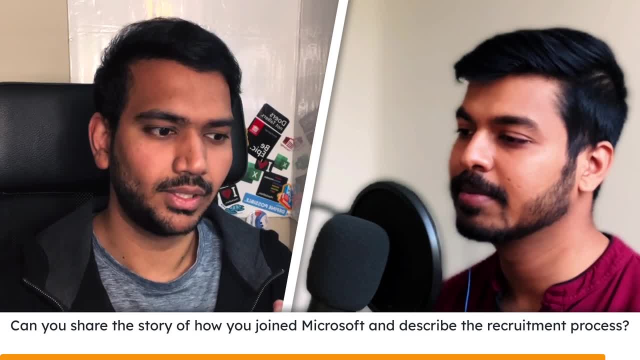 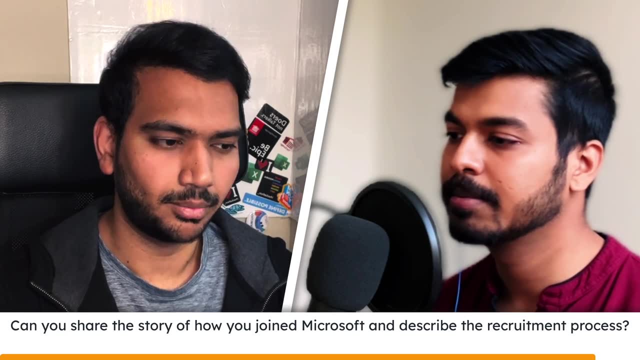 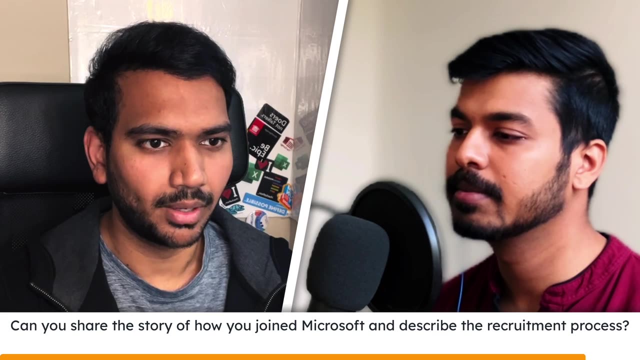 motto that i've ended up in the us. so, with that being said, i kind of like the way that microsoft works before that, before joining it, power to microsoft. i at least kind of understood that. what are the kind of uh things that they do? i mean, like what? 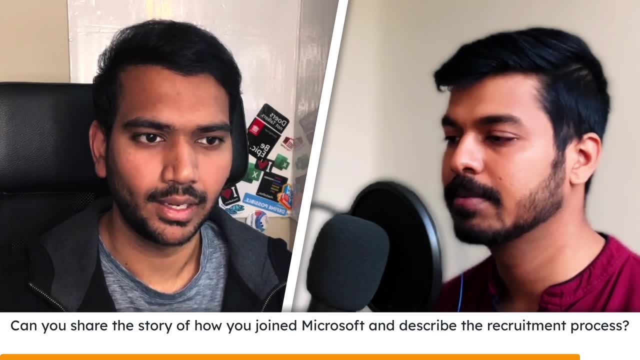 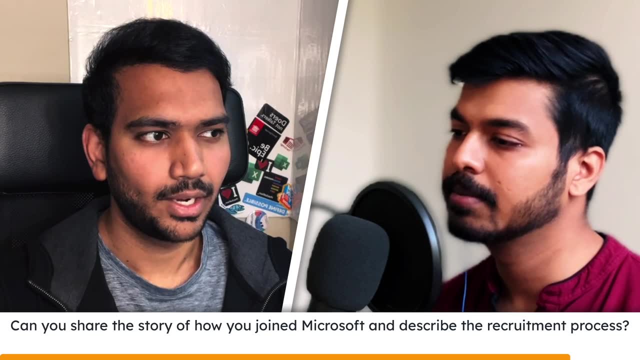 are the products that they kind of put into the world and like how would they actually had a shift between the leaderships over the last kind of 10 years? so seeing that, uh, i kind of have this sort of like soft corner that i could see with microsoft some for some reasons, and especially i've been 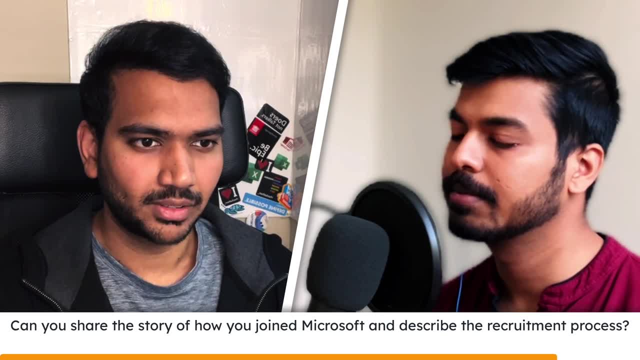 joined by a lot of people and i've been working with them for a long time and i've been working with them for many. microsoft- i could really watch that. this is the one of the best companies that you can ever work with because of the way the culture has been put among the people. it's kind. 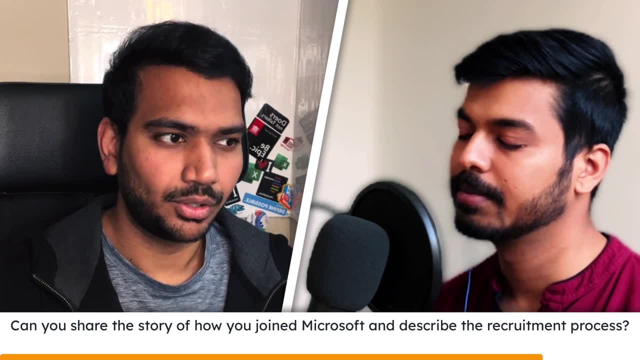 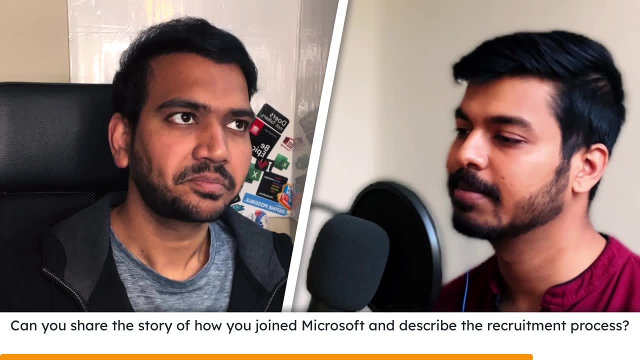 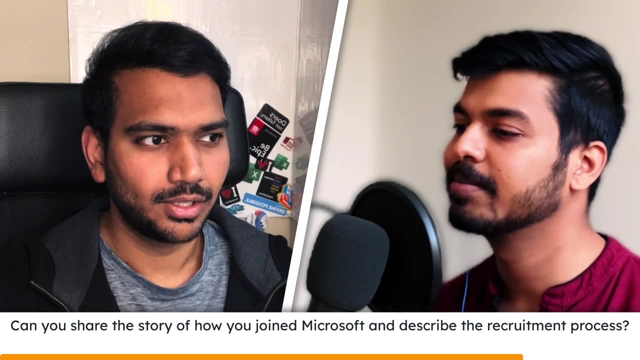 of. really, you know it makes you to, or wants you to go to the office daily and give something like productive kind of work, that is, human data. so keeping that aside, getting into microsoft was kind of hustling that i could say of, but like soon after finishing or like in the last semester or 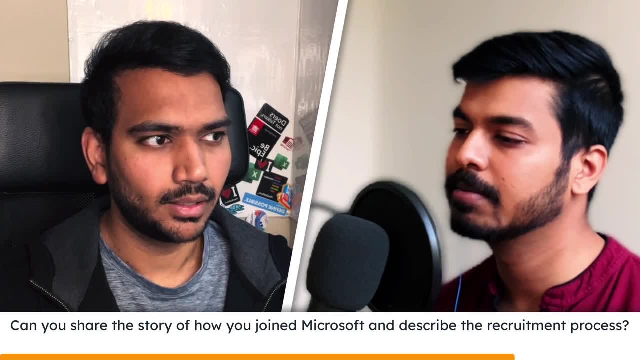 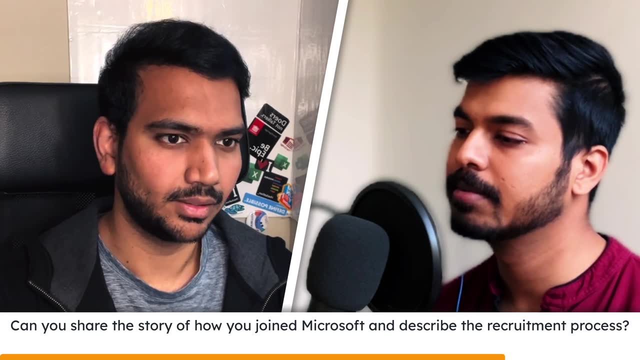 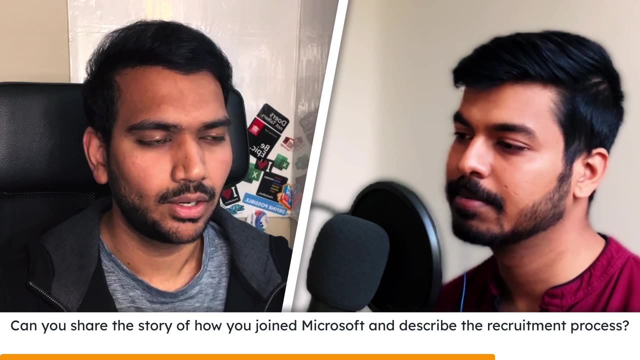 while of my master's program, i was completely searching for jobs, dropping emails, uh, applying for to carry the photons, among multiple companies asking for her fruits. it's kind of a hustle that i could say of definitely so. any on an average, any kind of immigrant student who would actually 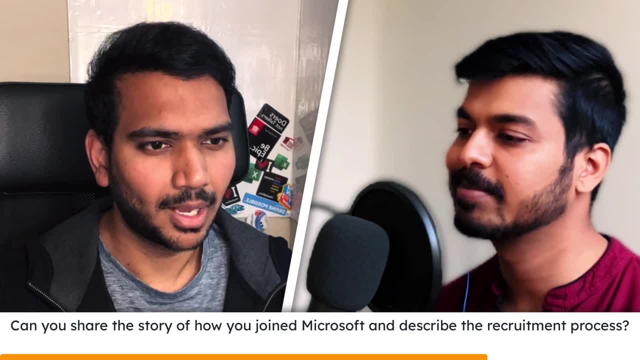 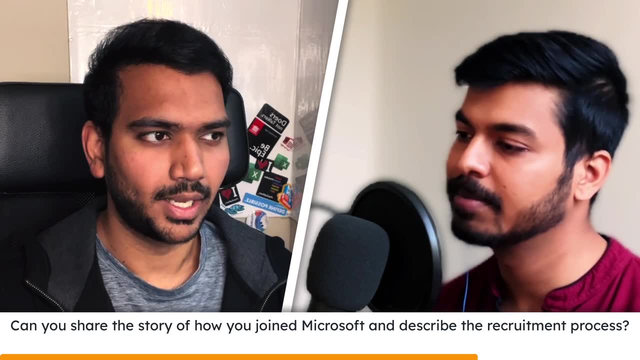 apply for at least four out of five hundred or thousand jobs applications. so that's the kind of thing. so you can kind of apply for jobs. you get rejections and everything is part of the game. and early in the process when you get calls from different organizations, at least from the bigger, 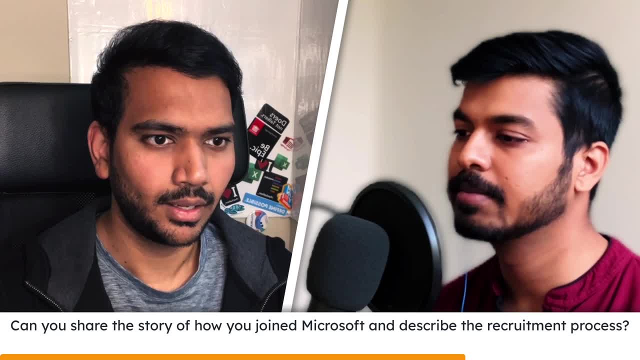 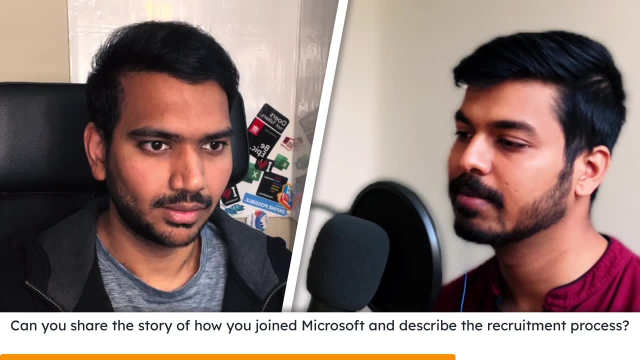 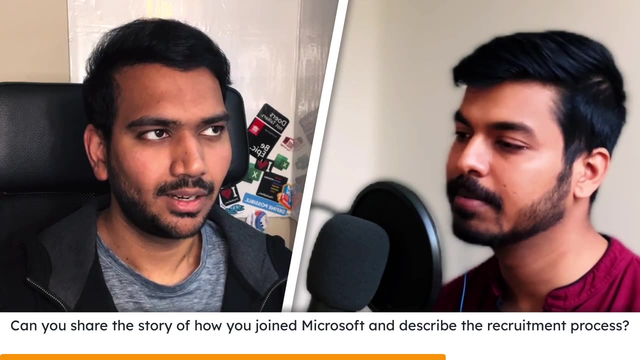 bigger organizations like amazon, google, microsoft, anything like that. you would feel that overwhelmingness as well and saying that, okay, am i right now in position? but interviewing with these big companies or something like that, it's totally fine. you need to be calm enough and keep going. well, i still remember that, giving my early interviews with all of the amazon's uh teams. 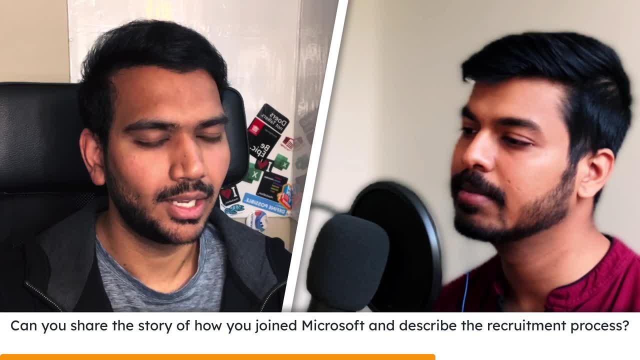 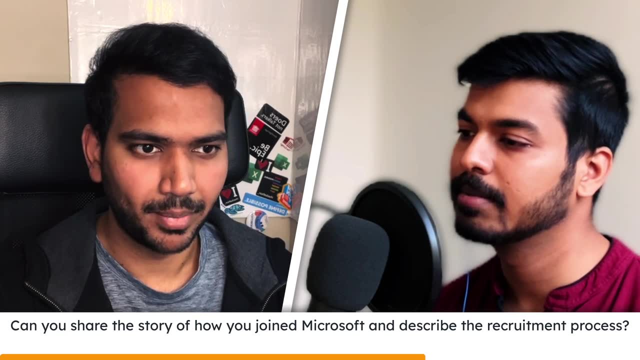 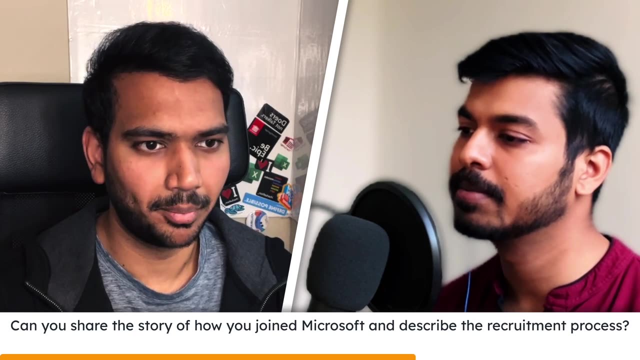 when i completely, uh, couldn't give my portfolio presentation in a very good way, and i really understood that, okay, i shouldn't like: where did i? where exactly i had made some kind of mistakes? how should i avoid that? how would i, like you know, improve myself for the next interview or with whatever company it is? so that's how i kept. 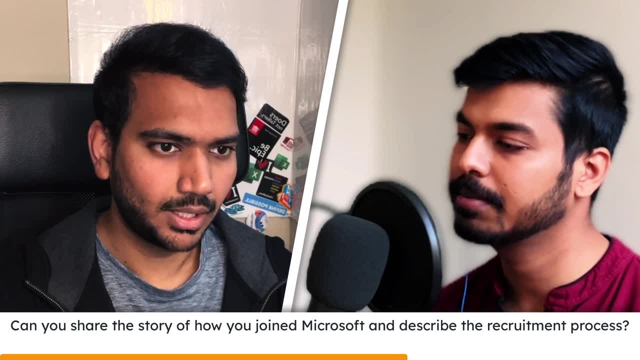 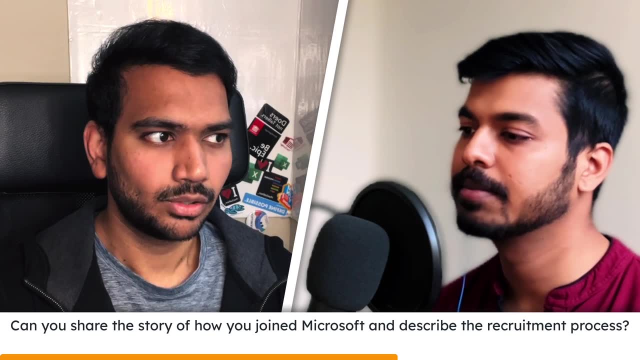 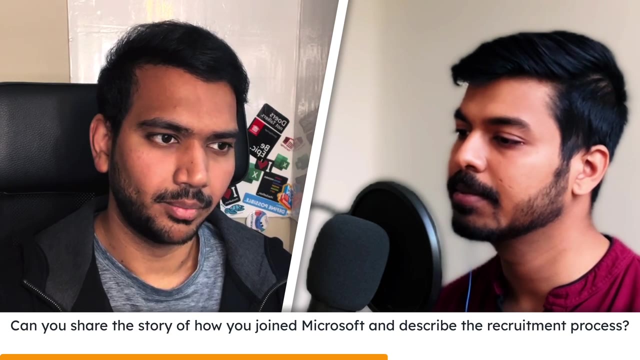 getting interview calls uh, preparing myself to that interviews, doing some mistakes, correcting it and somehow like moving the art. so before entering the microsoft, i had to be kind of the? uh. got a period with hyacinth, which is one of the electronic consumer makers i was linking to tv os. 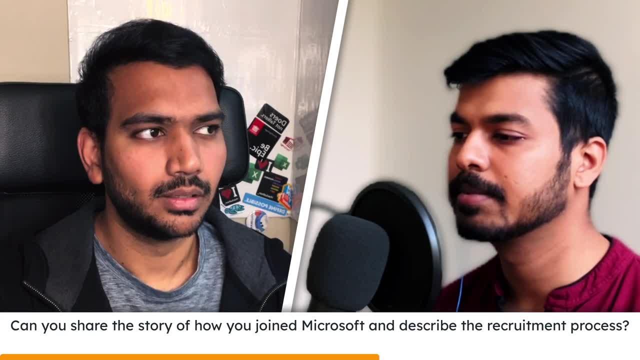 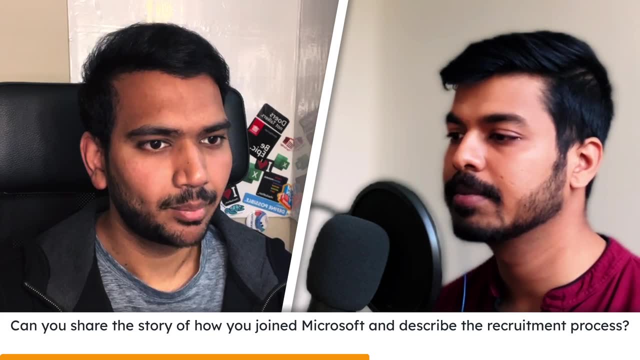 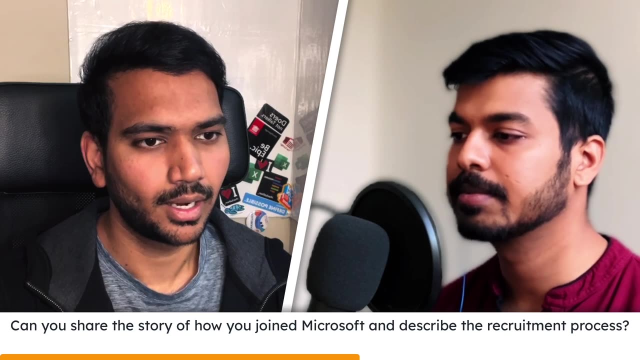 design side of it and i was kind of working with them. so even in that part of time i wasn't really aiming for a particular job with microsoft or any other big comp tools, but i kept doing like saying that okay, i'm not good to settle for a smaller thing that i'm going off like really work for. 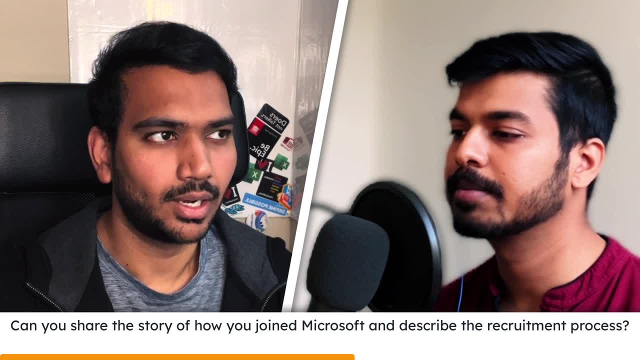 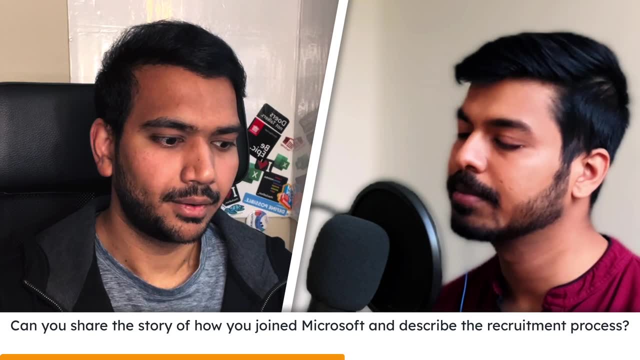 that. now i didn't want to. you know, empower on a big cloud, like at least work on the bigger products, that i could do, and i was like, okay, i'm not good at that, i'm not good at that, i'm not good at that. i could really empower many people on the globe, it's on the globalist, and i'm a kind of a person. 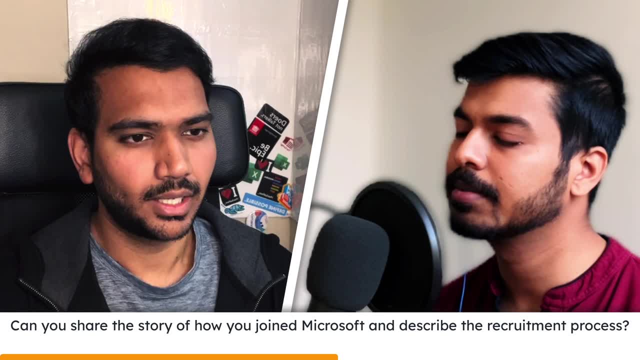 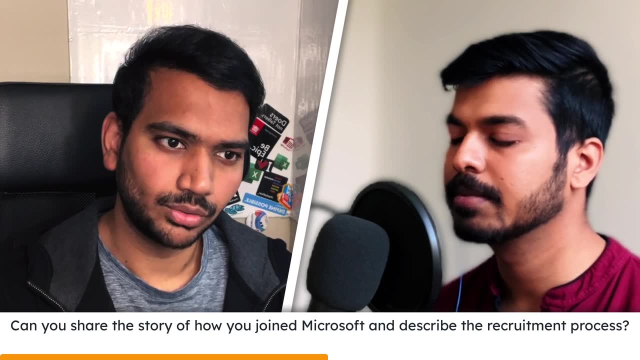 who actually looks for. uh, as i'm being in the early kind of phases that the caddy would like, ideally wanted that kind of guidance, or the outlet from other designers that they are outside right now, and one better thing is like these big companies don't have that kind of cultures, or 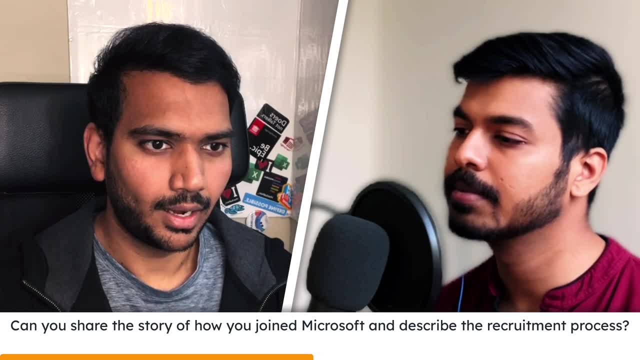 people right now, and then it's that. it's that we have to get in and we do. we need to make that connections so that we can understand the culture and the people right now and then we need to make that connections so that we can understand the culture and the people right now, and then we need. 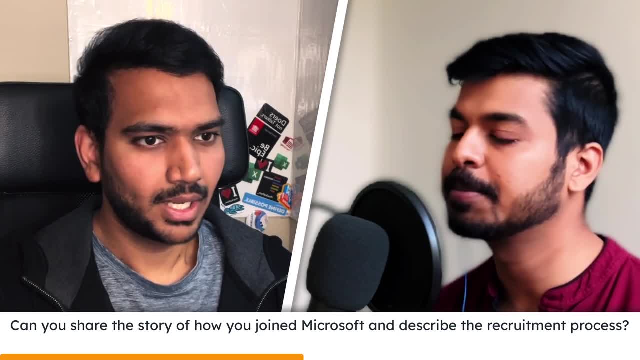 that connections so that we can understand the culture and the people right now, and then we need that connections so that we can understand the culture and the people right now, and then we need you know a little from them as well, so that kept keeping, uh, keeping me going on and uh, one i have. 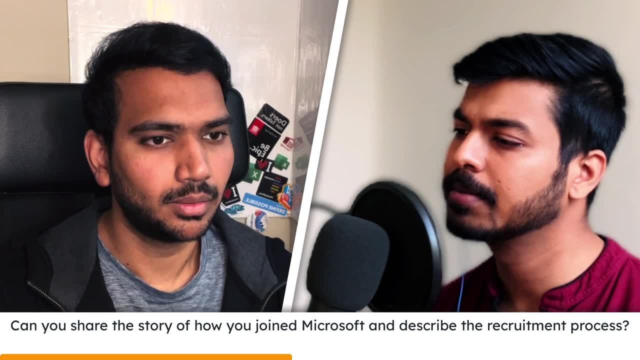 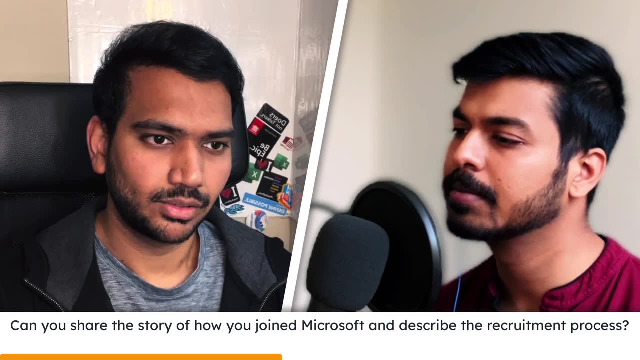 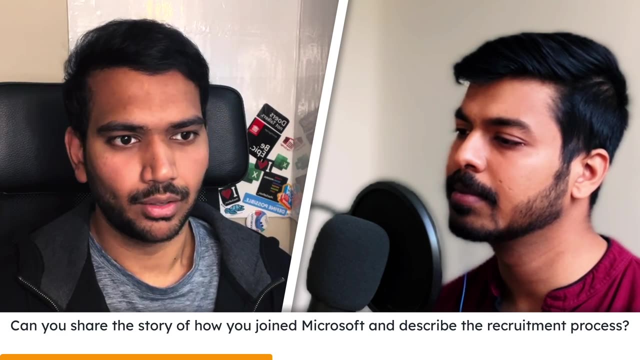 received, uh, like you know, of course, from different teams within microsoft. i was talking to their hiring managers and everything was fair enough, and one team got really interested in my background work that i was kind of doing and they kind of aligned their work with, uh, my kind of previous. 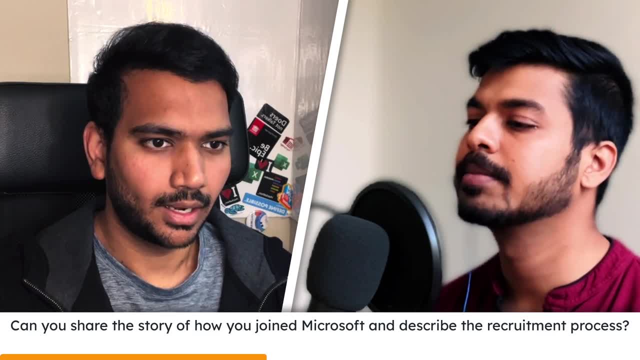 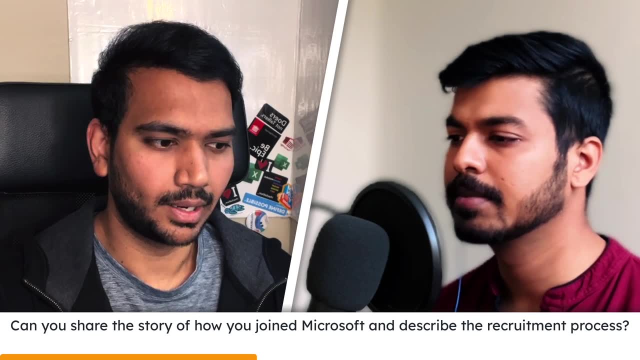 works, and that is why they have given me a chance to uh get an. actually do it so with microsoft it's kind of a straightforward process that you could see. it's kind of open again. i guess, uh, you'd be needing a one full date. they'll be blocking the one full day. 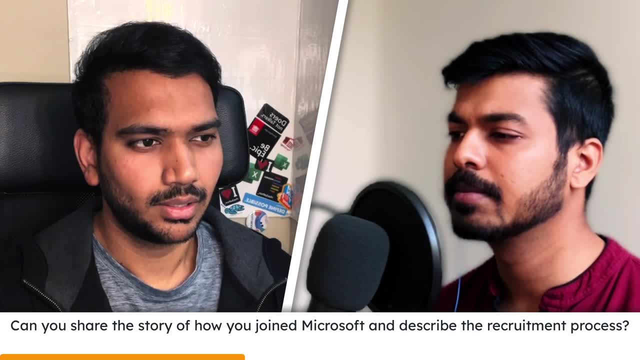 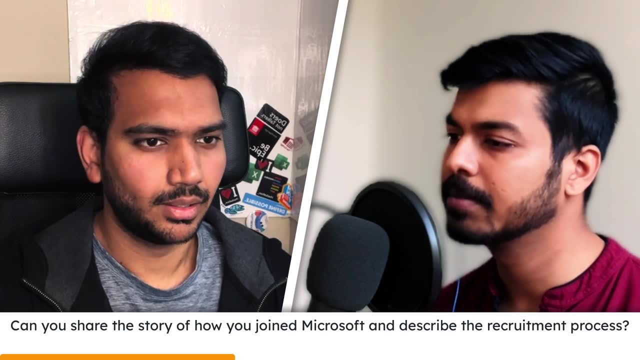 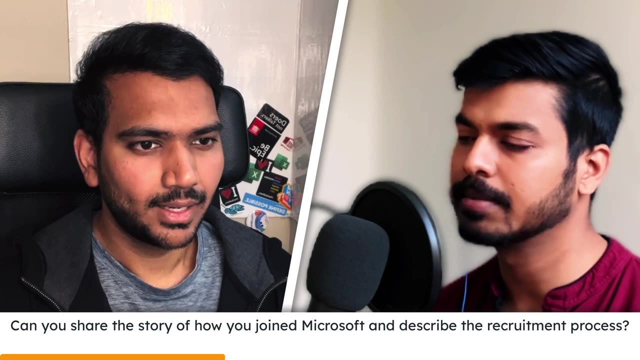 and giving uh like they'll be assigning you with different kinds of calls. uh, we'll be having four to five calls with uh different folks like senior designers- uh, for designers, i'm like principal product designers and our director level calls. so then they're understanding that, see you as a person and how would you present and like, how would you work within the team? 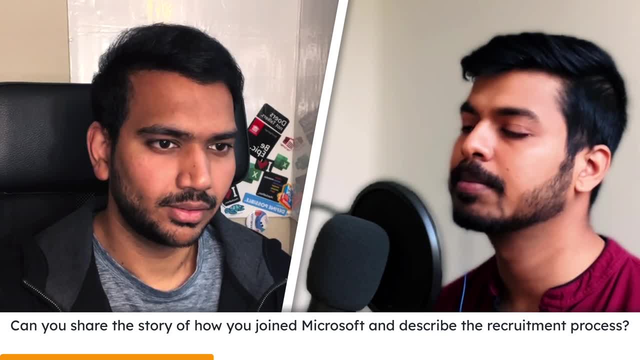 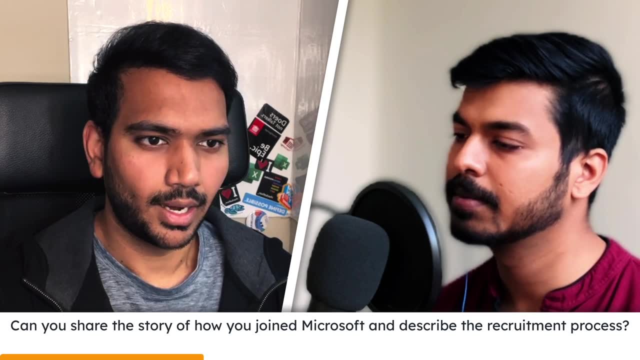 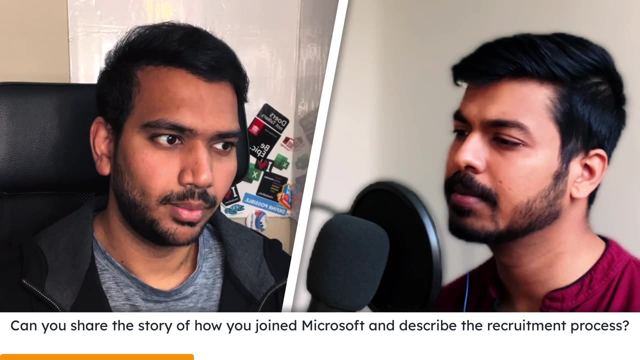 you'll be having all sort of like behavior analysis questions and your previous internet, previous kind of works that you could present to them and everything as such. so that is more of an analytical and like strategy thinking that you could put it into those interview cards and at the end of the day or any time in the day, you'll be having one hour kind of. 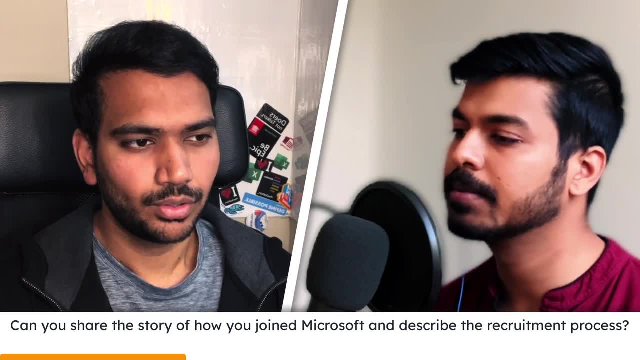 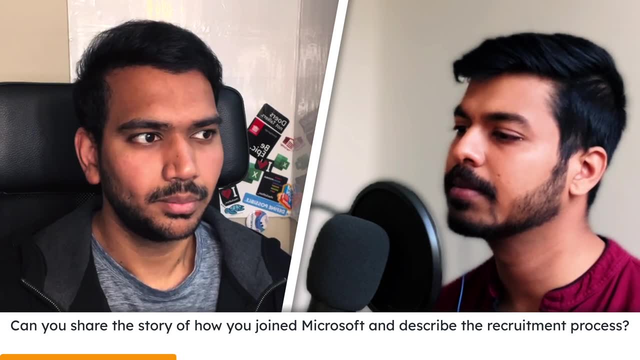 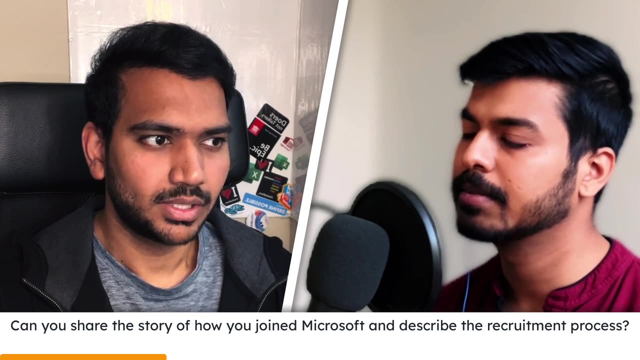 portfolio review kind of session, when- and this portfolio review session is something that the candidate would try- the whole portfolio review session and the candidate would try the whole whole session. uh, and we need to align the time exactly and you know, so we need to present, like, at least three product uh, three uh works that we actually worked on, green risk works, which can. 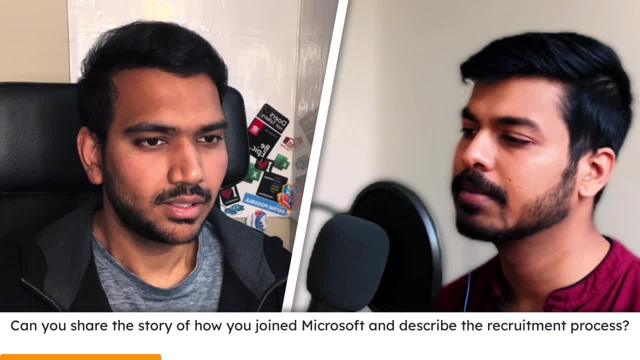 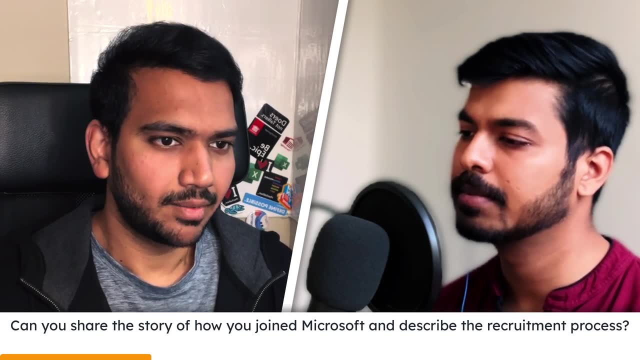 align with that particular team and you need to manage the time so that you'll have the last 10 minutes for qna session and you need to keep going for the entire session. it's like we're driving it properly and they would be seeing that okay and they would be analyzing, like how exactly is this? 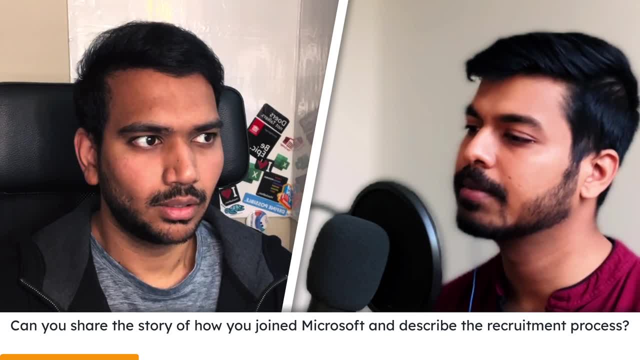 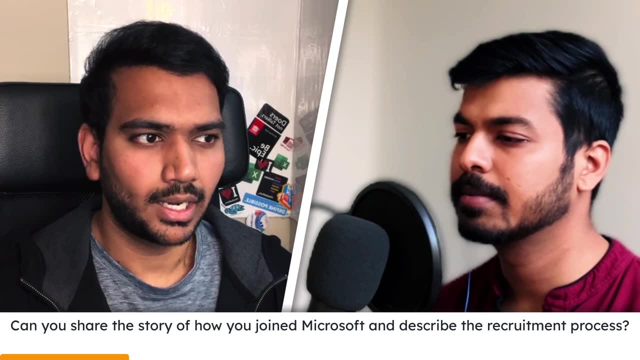 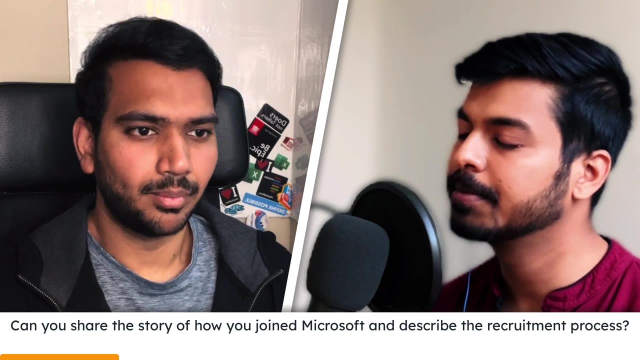 candidate driving the session and, uh, you know, keeping the product relevancy around it and answering the questions in the right way and how would they take a negative kind of feedback or a critic kind of thing towards a positive side of it? so they'll be analyzing everything in the back. 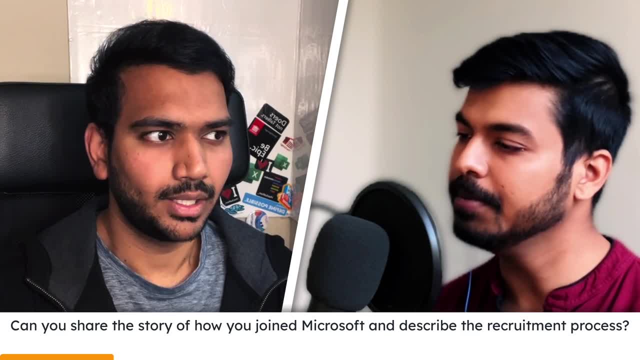 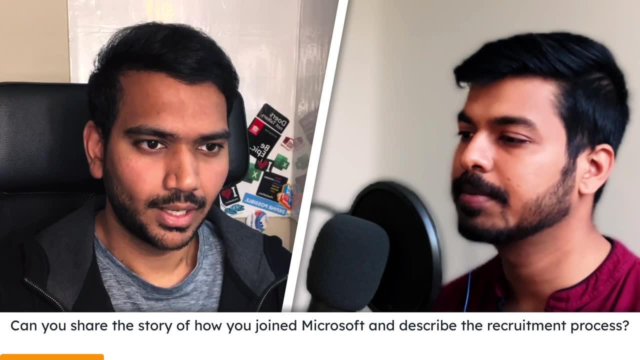 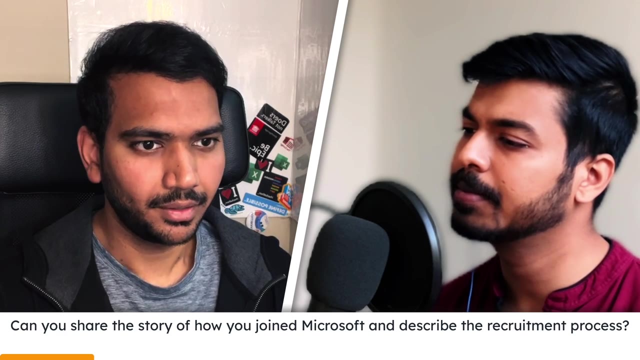 end. it's something that we need to be ourselves and we need to show an attitude that we'll be learning, uh, and we'd be interested to learn from anything like that. so it's like a genuine connection between the team with everything, and there's a candidate that we need to feel so when that right momentum is created. uh, that is. 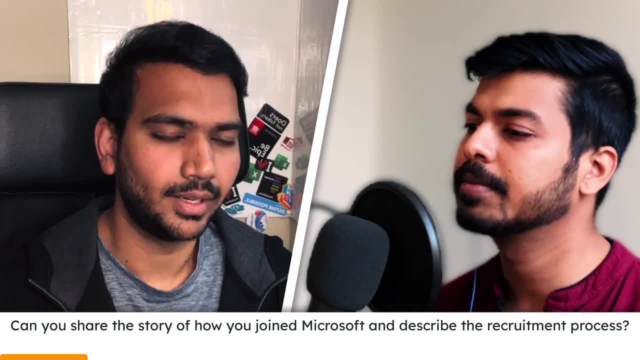 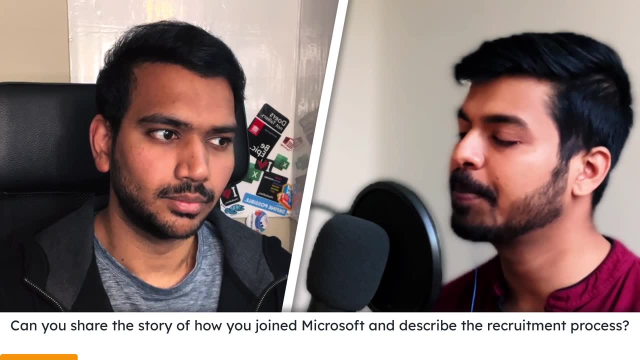 when kind of get into the, you know, we kind of think that we just leave it in itself. so that happened. interestingly, that happened with microsoft, uh, this particular team and uh, yeah, uh, they would feel that i'm the right candidate that we need in that part of time and, yes, that's. 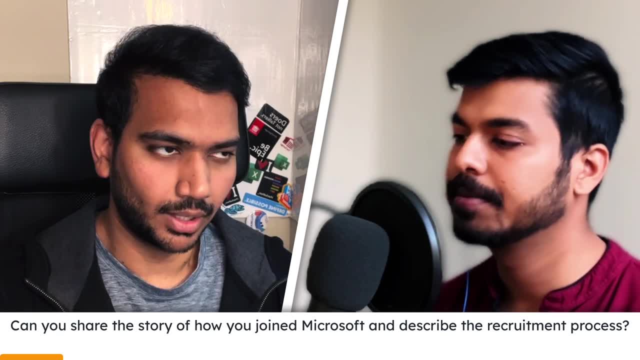 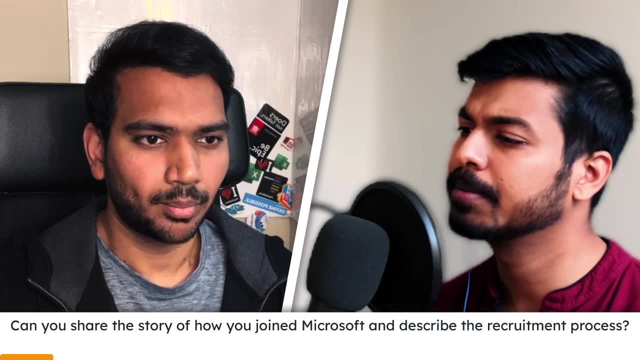 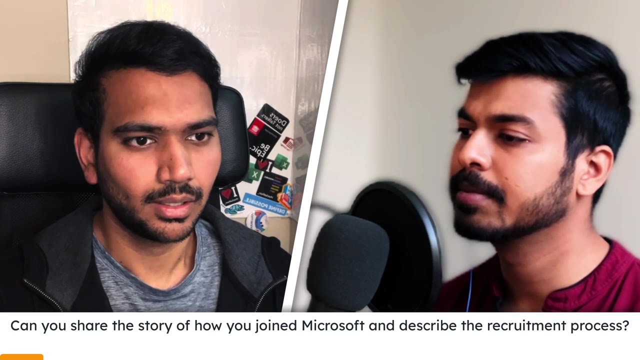 like i got a chance to get, though, into working with this team and one big thing that microsoft. Microsoft restricts you to apply to a couple of applications and wait for the next three months so that you do not hold it back with those kind of things. 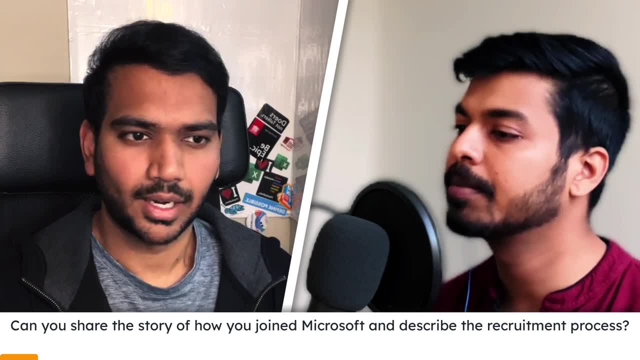 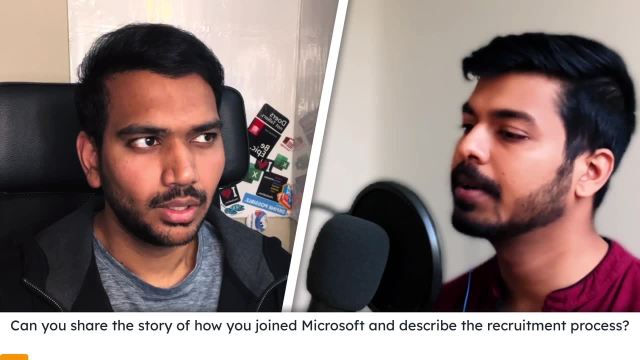 It's like different teams function differently. if it's in Microsoft and it's kind of open that you could apply for the right jobs that you find it in the career portal itself, But with Google, what I've observed is they do have this restriction of two applications. 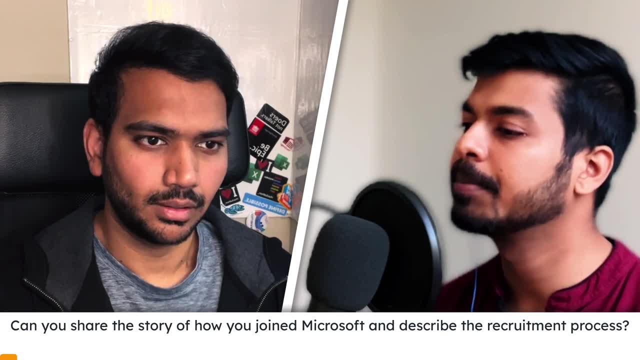 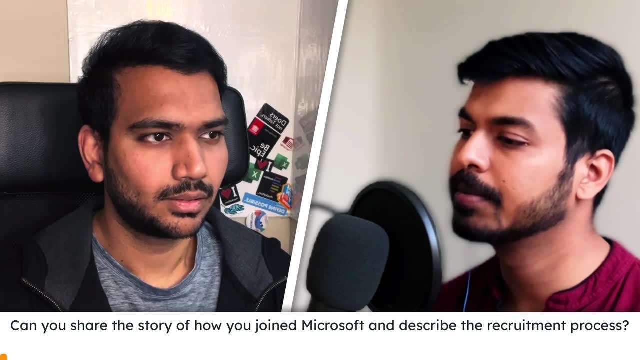 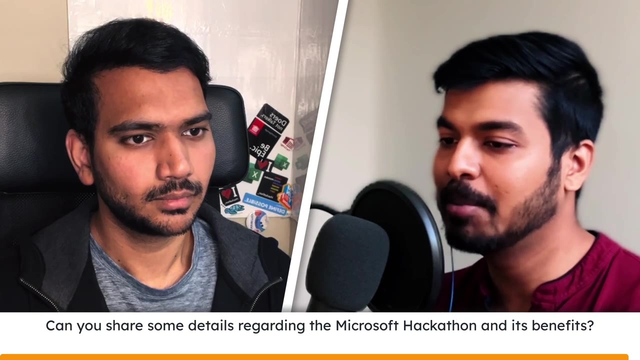 for a certain duration and then you have to wait for another few months or something to go back. Same is the case with Meta as well. over the years, This complete scale recruitment process kind of works in a different ways that I could say. I have basically seen that you have been part of a Microsoft hackathon and you also 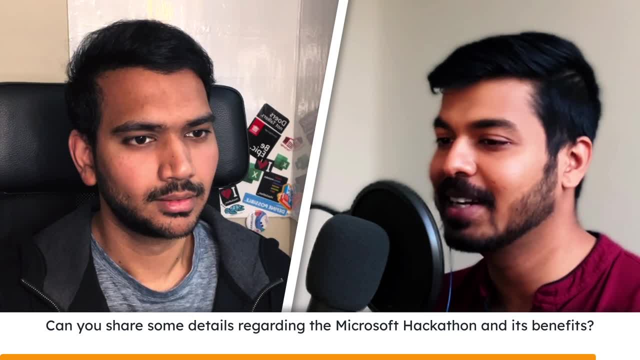 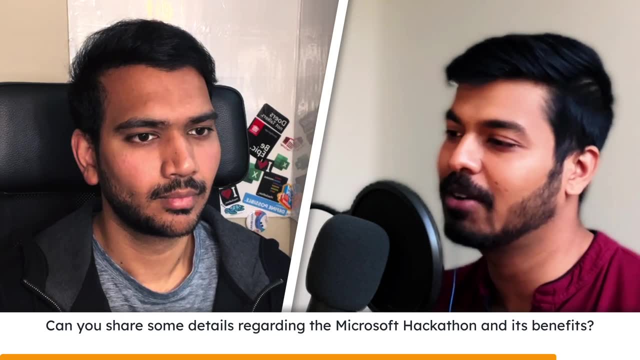 won it. So I was seeing this as a couple of posts on LinkedIn, So could you like tell us a bit about it and how one can participate in such things, and also, what kind of benefits do you get? How do you have participating in these? 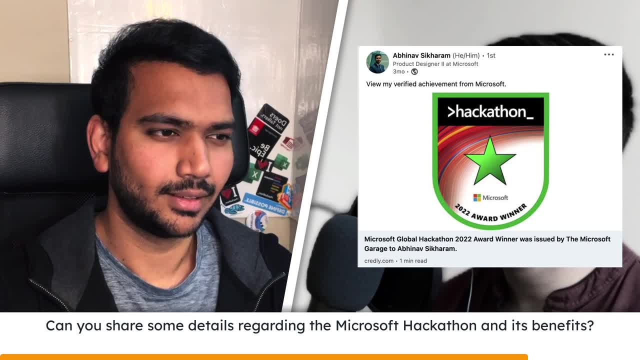 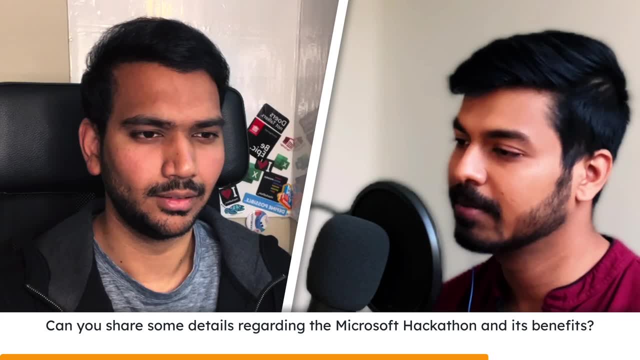 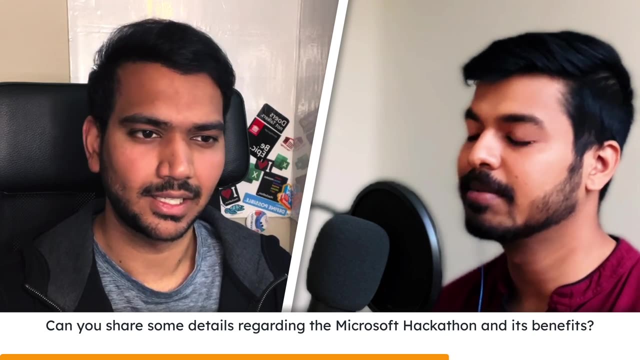 Okay, Microsoft hackathon is kind of an interesting thing that happens every year to support them. So this was the first year that I kind of jumped in and, like you know, was trying to understand the three pillars within Microsoft. We have these garage facilities for Microsoft employees that we can actually get out of. 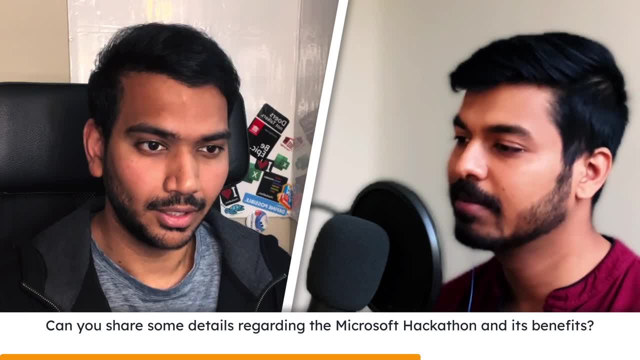 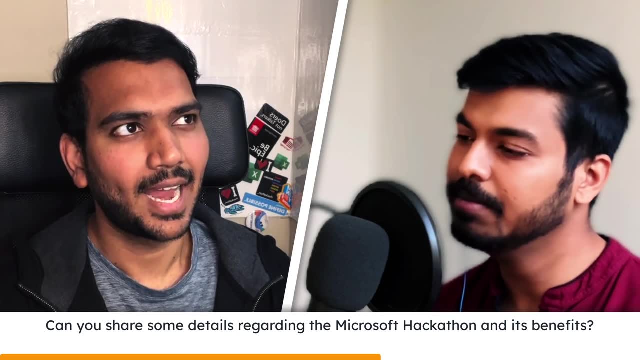 the regular jobs and actually try new things and learn new things as well. So that's a great facility that people have. So it was. It was one of These challenges So we had. There is this global challenge that some of the team has actually won. 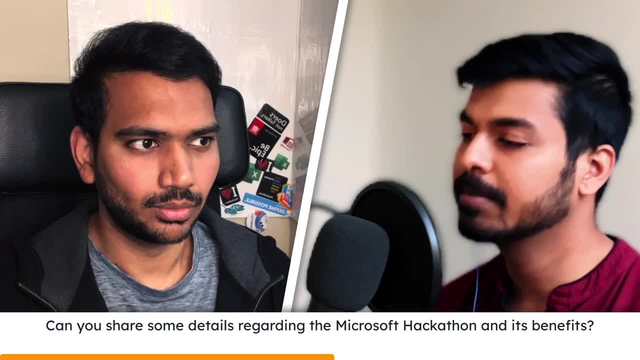 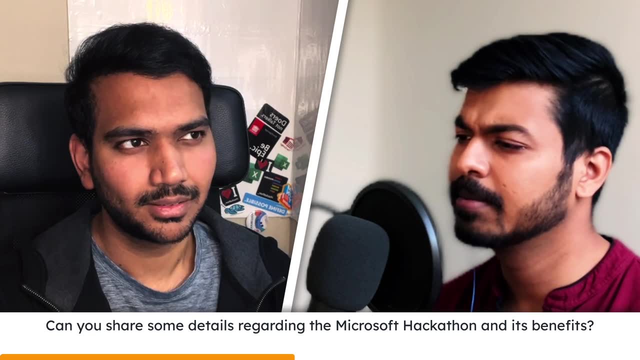 Like I was one of the winners- based in Atlanta City. So then I'm like multiple challenges within the hackathon and it's kind of the major. the actual winner is based sort of in another place. that I couldn't really reveal with idea policies. 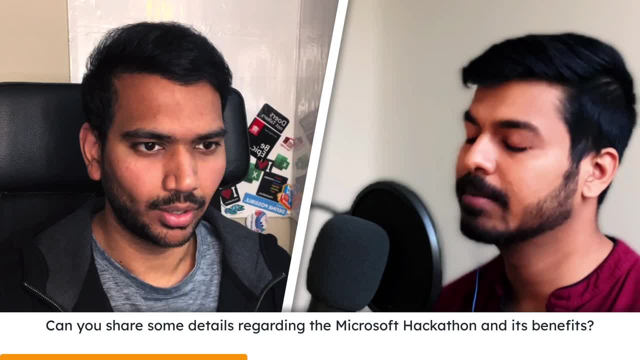 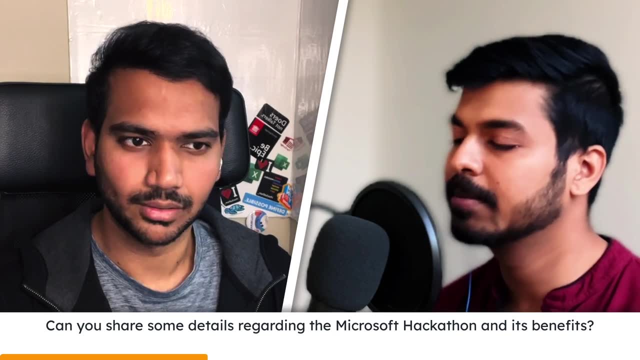 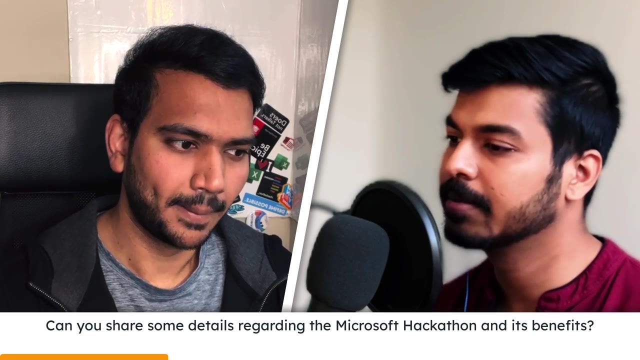 Yes, We have these hackathons every year happening for employees for a week duration and it kinds of gives you the opportunity to you know, Puzzle with things and to learn new things or like explore new things, anything in that, or if you want, to the improve certain areas within your product, you can do that as well. 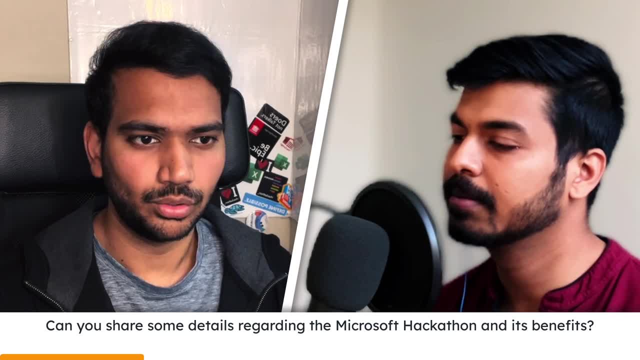 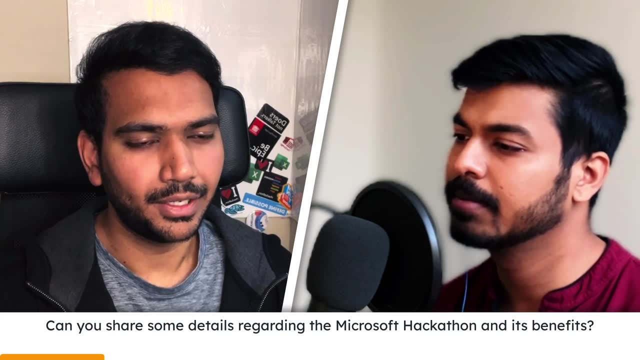 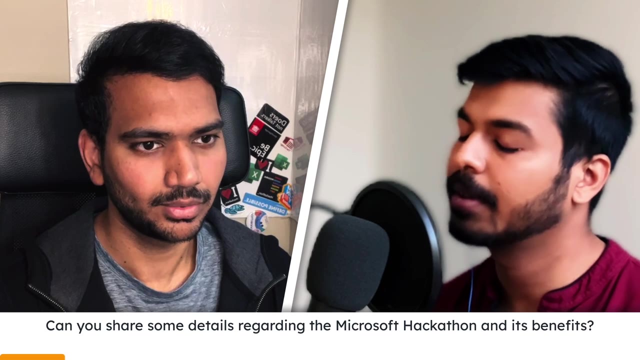 So it gives you the flexibility and opportunity to the employee to do whatever and, you know, to make itself more exactly that they have. But yes, it's kind of an internal thing that happens every year and I think external participants cannot participate, for within our hackathon programs. 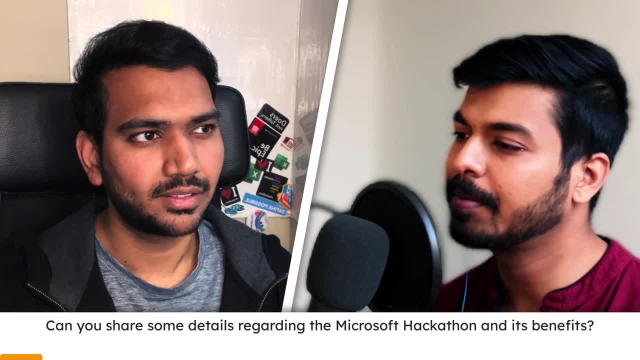 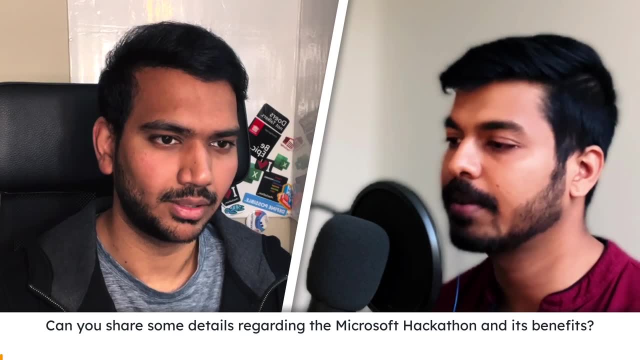 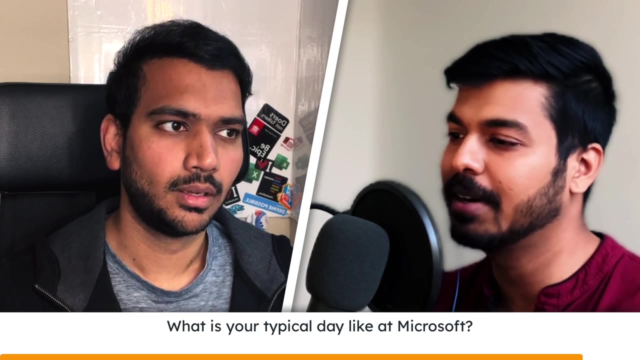 Like- And yes, it's kind of a knowledge learning or sharing kind of thing, that whole wheat is kind of encouraged for every other client. One last question, Like: how is your general day to day work at Microsoft? What do you do on a day to day basis, on a typical day? 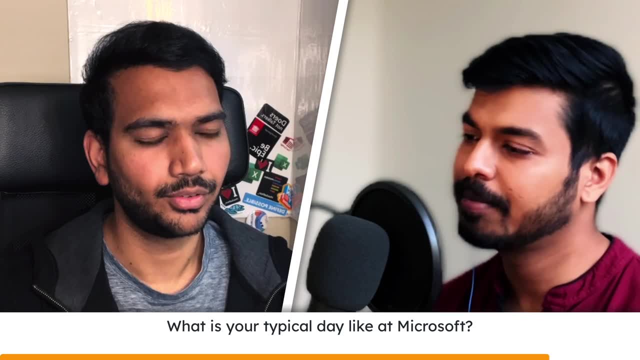 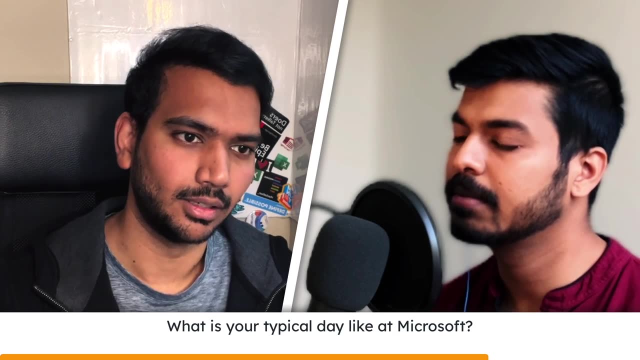 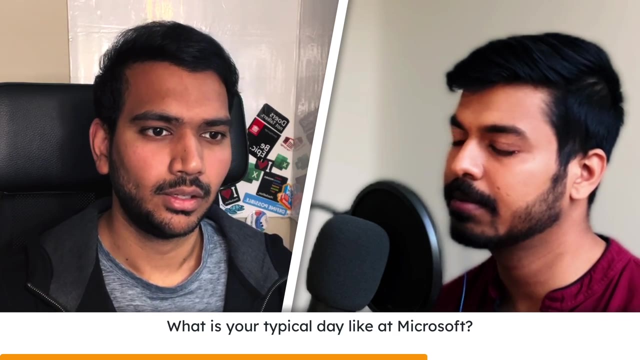 On a typical day. it's kind of we work on different features within the product. that I could say often like we need to make sure that we can do a PowerPoint and, like all together, align with the users. There are a few features that we did here. 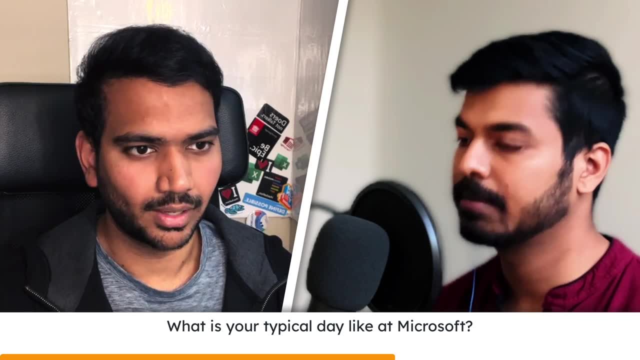 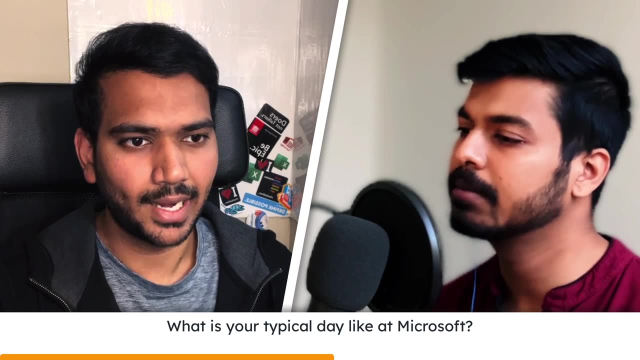 So it's like a lot of collaboration happens between different designers and researchers. that I could say, because it's kind of a we sit at the product level but at the same time we need to be in tandem with other products or the system parts that they could see in. 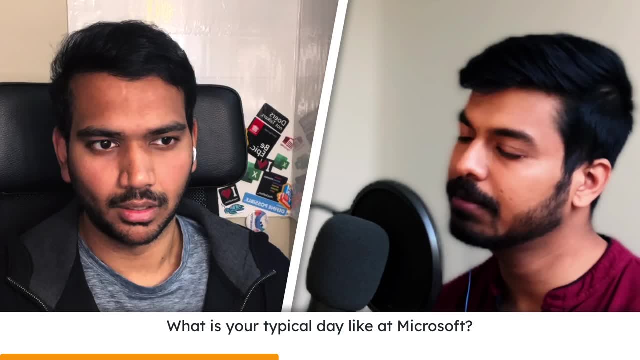 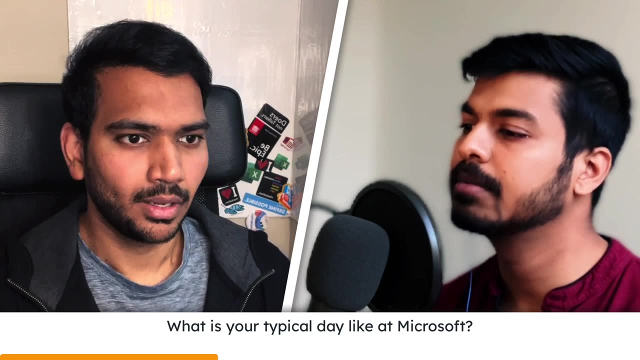 office apps. So on a day to day basis, I do collaborate with a lot of people across the globe, Like I collaborate and like work with teams based and PMs based in India and there are a few people based sort of in Israel and there are few people based sort of in Thailand. 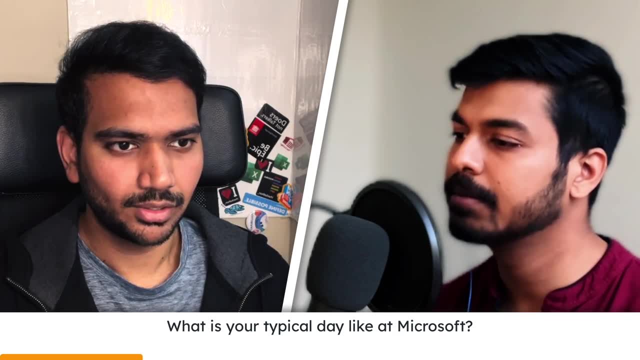 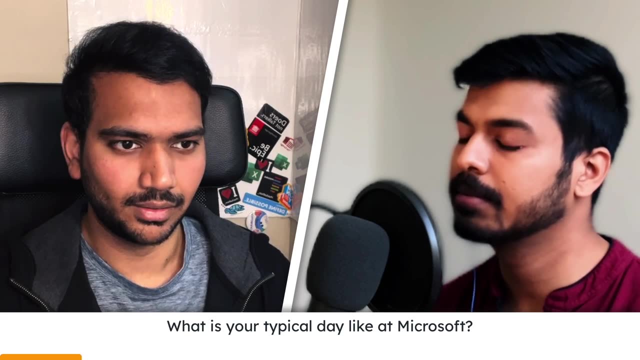 So it's like a global team all together and it's kind of a diverse team that I could say of. We collaborate a lot amongst the PMs, engineers and the design system, our designers, who actually meeting the design system like fluent design system that we have. 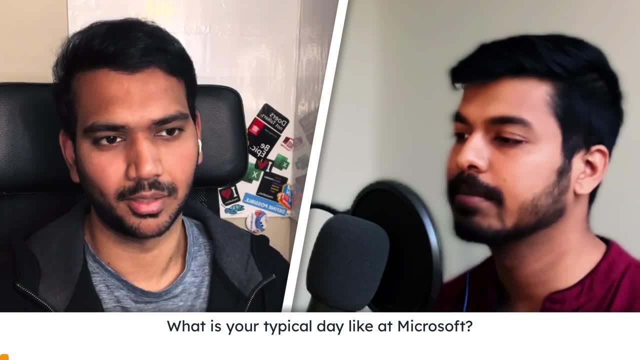 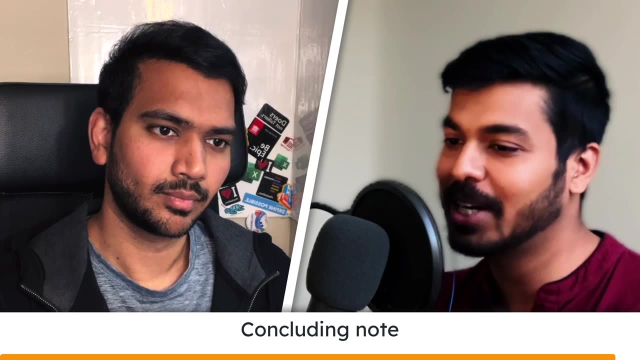 So collaboration is the key on a day to day basis that I can say of. So let's conclude this talk like on a conclusion note. I want to ask you like: do you have any tips or advice, Advice that you would like to share with the budding designers here? 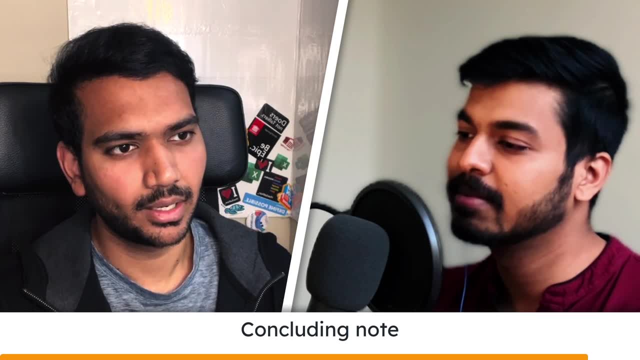 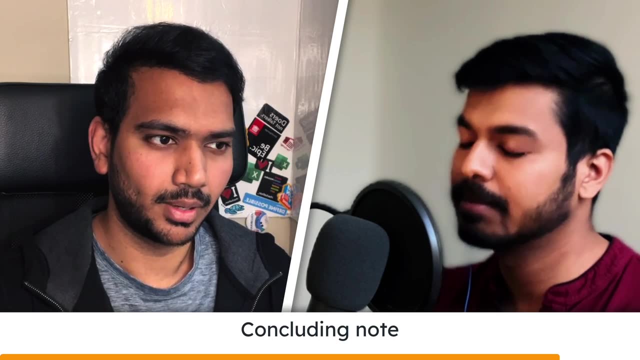 Right, definitely What I learned from my journey, like when I kind of recollected from the real, from in, starting from 2011,, like inserting and like come to the more, coming to the masters in 2019, and finishing it up in 2021. 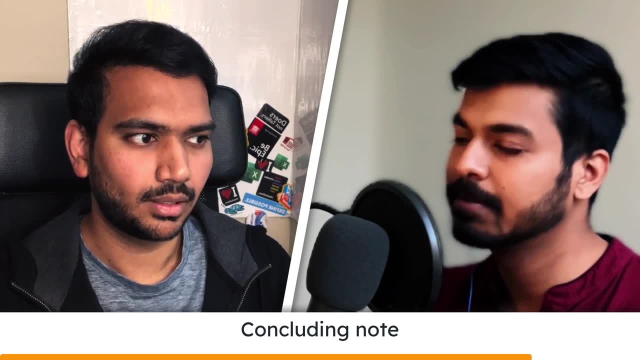 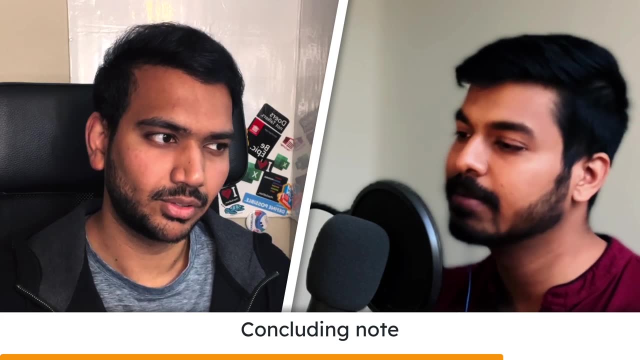 So it's like a journey of 10 years. So all of these, all of and all of these points of time, like I kind of missed the opportunity to get into IDC, I had to bomb it. I did really miss out the opportunity to get into NID because 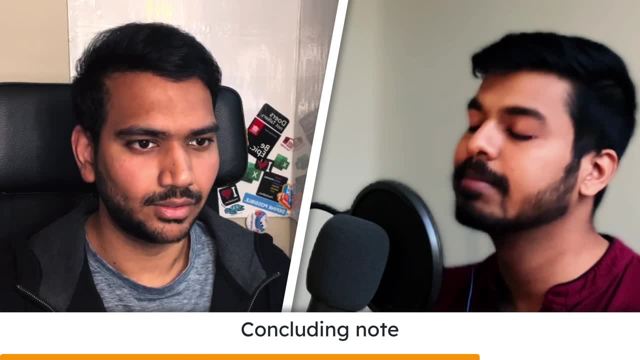 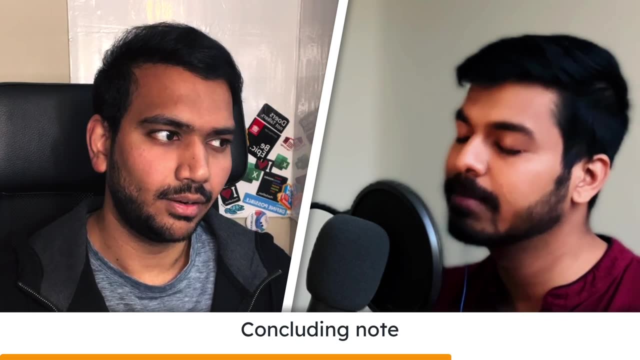 I got the seat in NID, but I had to take the decision of either just corporate job in Cognizant or NID. So it was a hard call at that time as well. And then I had to step back and I did really want to, you know, go to a job, understand. 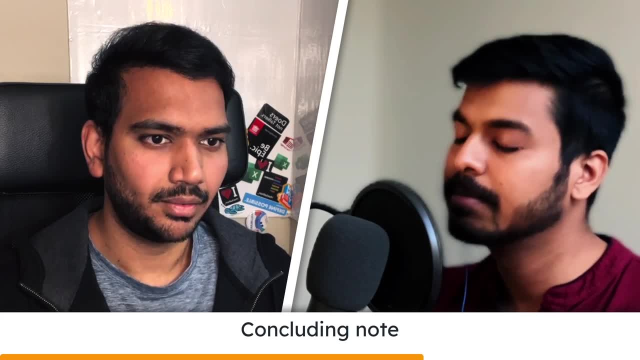 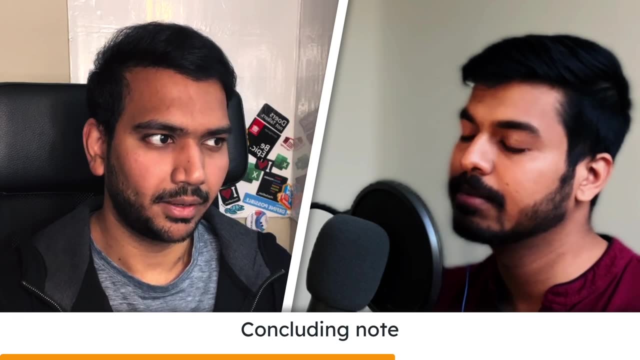 what is happening in the organization level at the same time and the industry level, So that gives me more exposure to what I thought. And then I waited for another three years, worked over there, then I came to the masters. So reconnecting this all of journey. 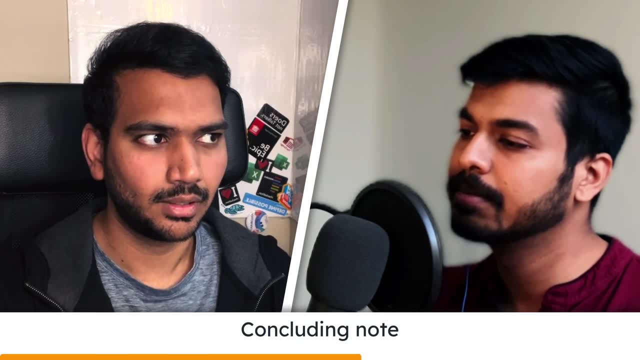 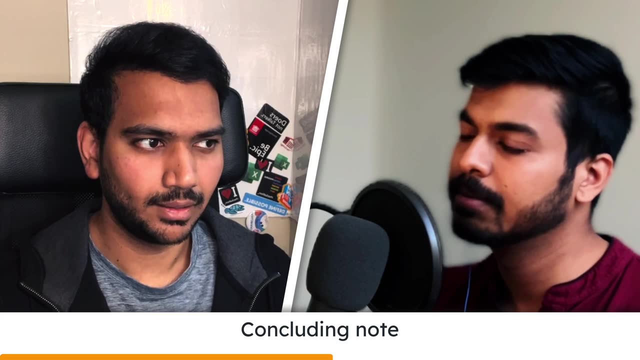 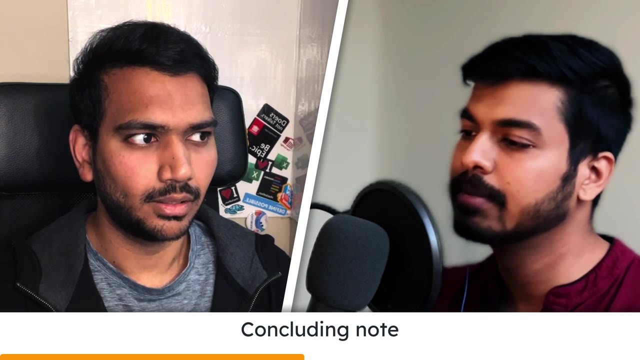 One thing is for sure: like I have this, you know I never wanted to leave this passion or whatever the idea of design. So I always wanted to be in that kind of learning side of it And I'm still really focused to learn things like it needs to be a learning process, a. 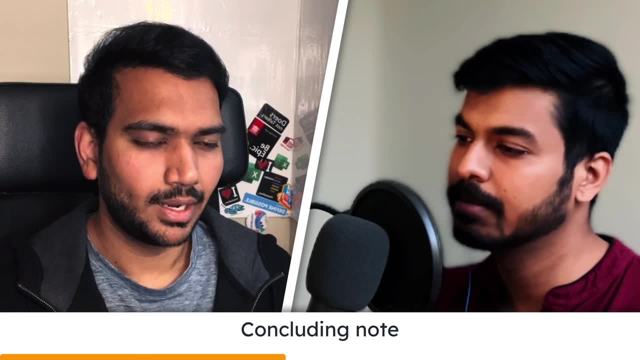 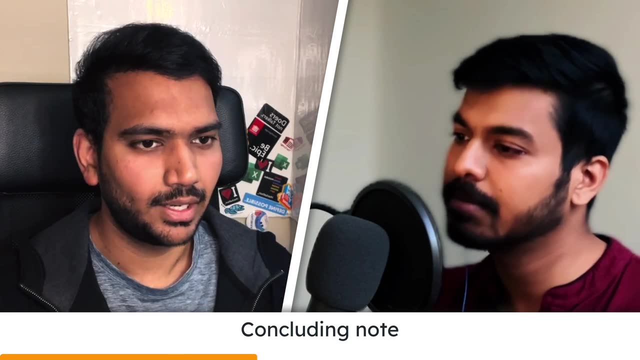 constant learning process, But in case, as a UX designer, you can't lead that learning And you need to keep growing. I am like you know. you need to keep iterating on a day to day basis. We need to learn a lot. we need to understand where we actually failed. 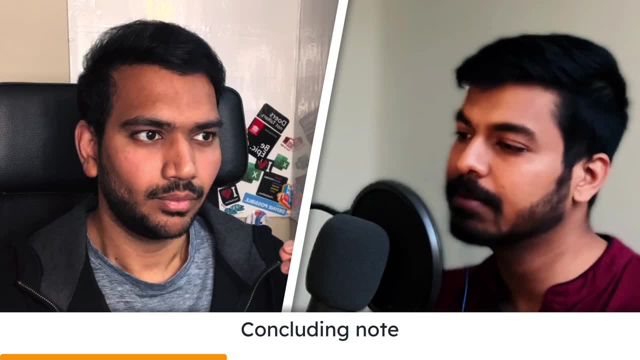 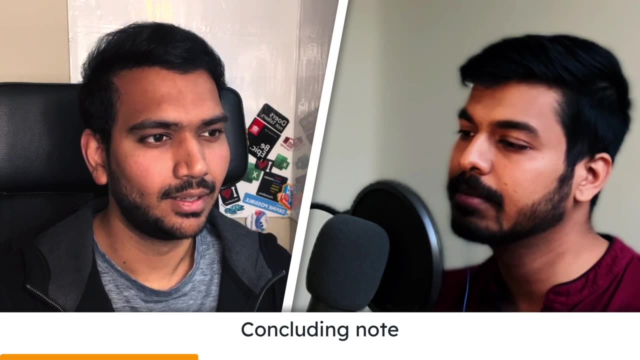 And we need to take that feedback. we need to think that critic we can be, it can be overwhelming. Definitely, on a day to day basis it will be overwhelming It. at times we feel that I'm doing exactly what we want to do. 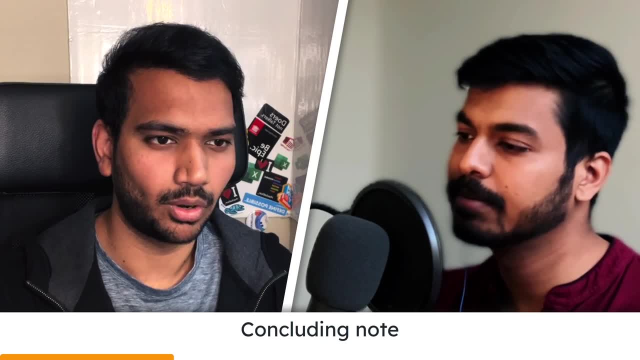 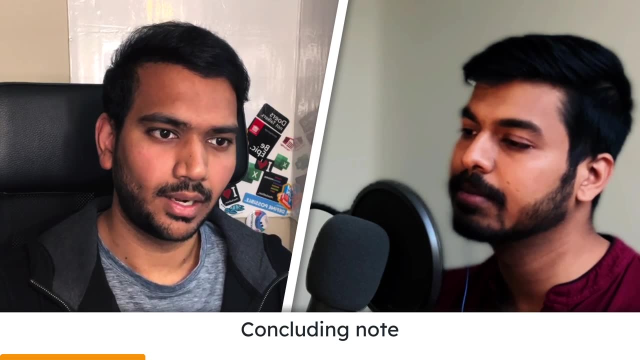 And, like you know, are we kind of in a productive, creating the productivity or whatever it is we go through. a lot is what I could say, but still, at the end of the day, the learning that you take out of it linked to the whole journey. 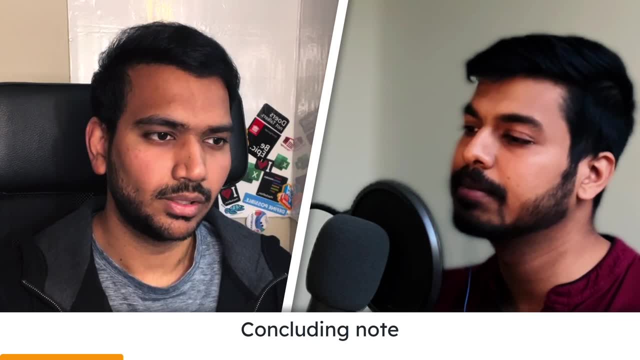 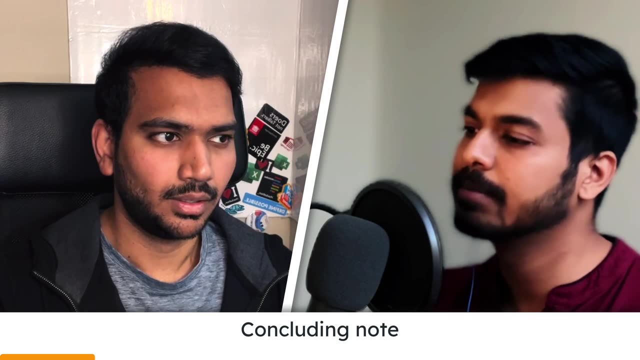 That really does matter. So the moment that I'm kind of going to solve the offer at Microsoft, that is when I recollected saying that, okay, whatever I was learning from the last 10 years, like you know, trying to get into the analytics course, trying to figure out if I'm really accustomed to design- 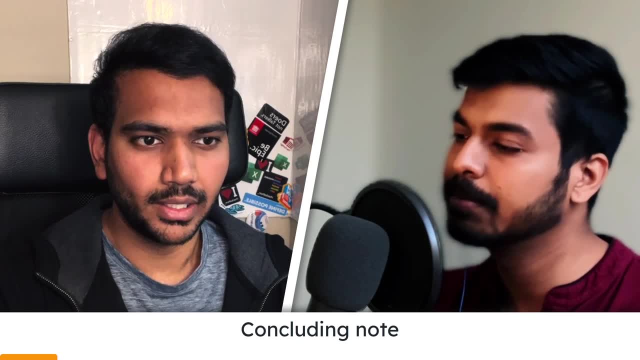 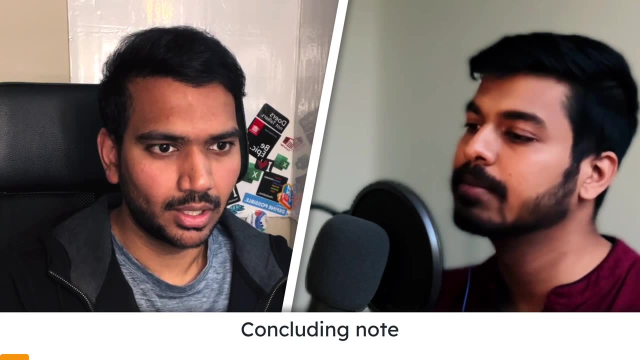 getting into those interviews at IIT. So even those small learnings that you would carry for at each and every point of time would actually benefit you at any end of the point of time in your life. So just keep on holding on to that core things that you really want to do. 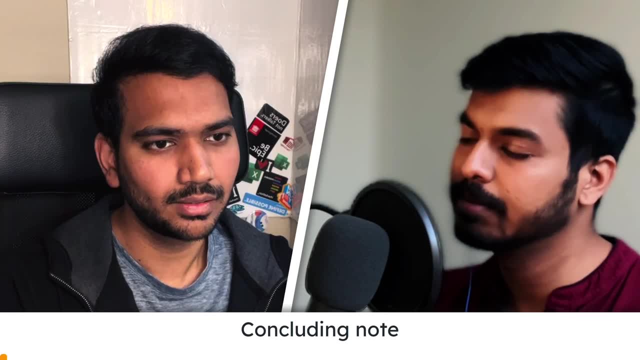